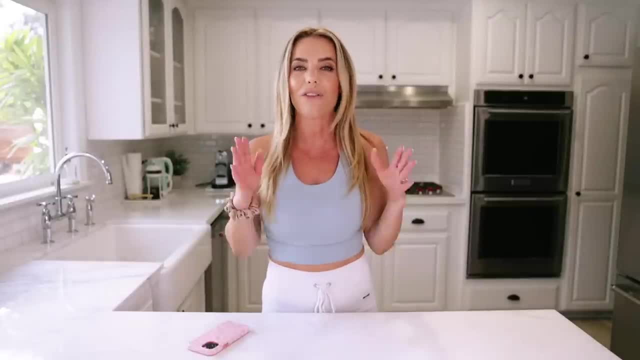 yet You guys, I have so many videos like this with more tips for you If you are on a weight loss journey, if you're trying to transform your life and get healthy, like I did. I lost 45 pounds. you guys, I'm with you. Make sure you subscribe so you can check out those other videos. But right, 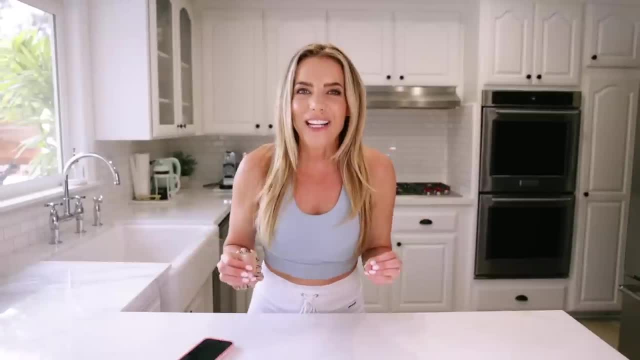 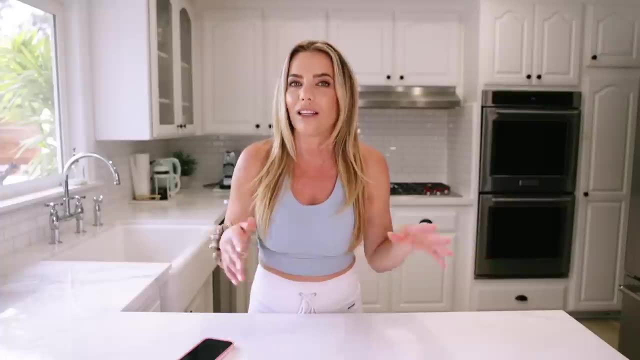 now let's dive into these 10 healthy food swaps. Okay, quick note on all this stuff too. It's all from Albertson, So it's just like a normal grocery store. Most of it can be found at like literally any grocery store that is near. 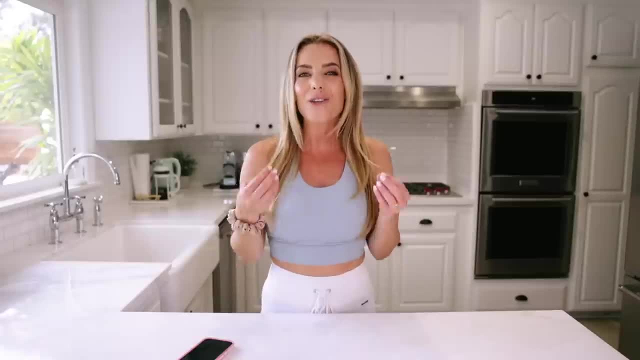 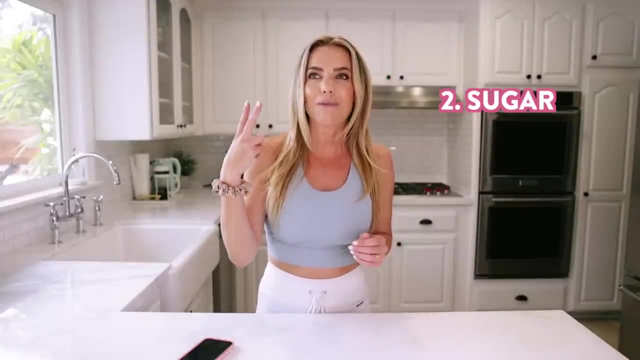 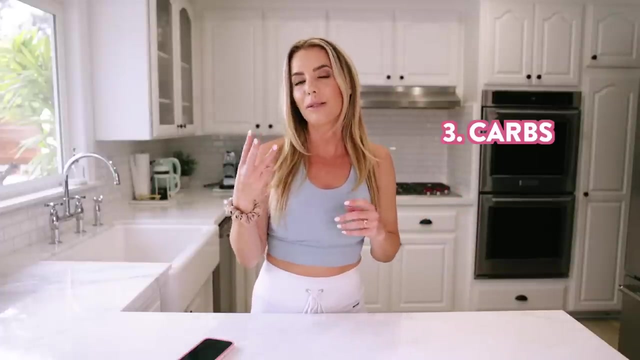 you, It's not a specialty one like a Whole Foods or Trader Joe's. And also, when I'm looking at labels, I look at a couple things. One, the protein intake. Two, the sugar. So one if it's like natural sugars or added sugars, and then just how many grams of sugar it has. I look at carbs. 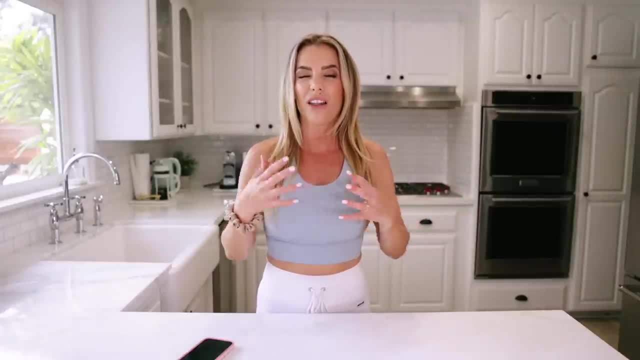 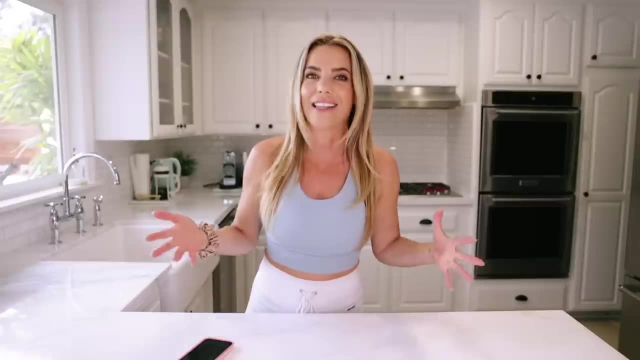 but not at how many grams of carbs really, just more The source of those carbs, like where do they come from? And then always at the ingredients to see like what's going on? Is there a bunch of added stuff that you don't need? So that's kind of how I. 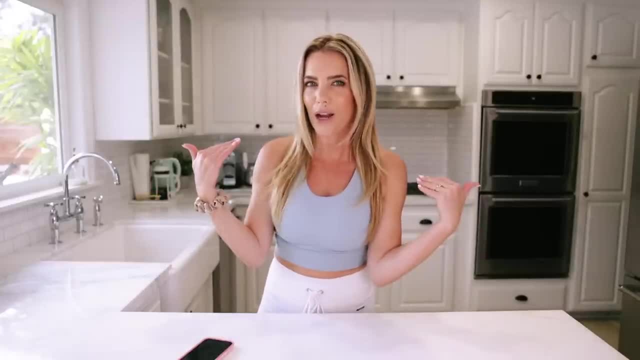 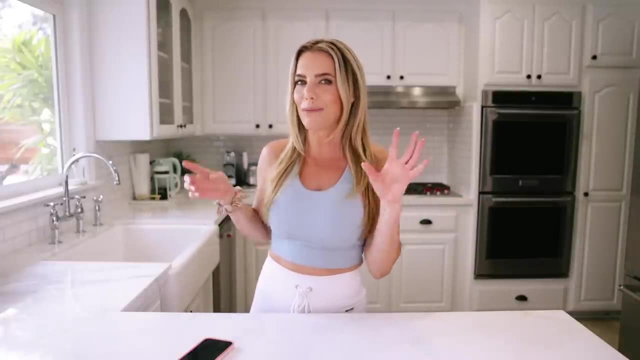 judge if something's like good to go or like a no go. So the first thing is one of Ryan's favorite foods in the entire world. It's one of mine too. I use it multiple times a day, but not this one. I'm going to show you like the average one. first It's peanut butter. This is just Jif, which, by the 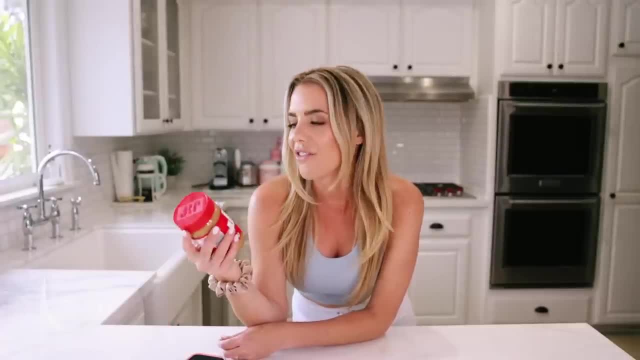 way, is Jiffy a brand? Is that what I call it? I'm very confused right now, Cause I've always called it Jiffy, And then I saw this and I was like it's Jiff, Are there two? 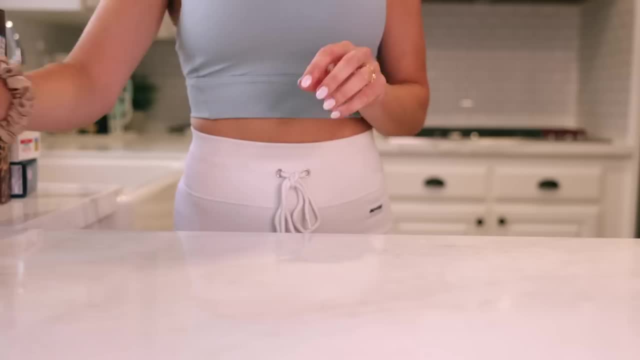 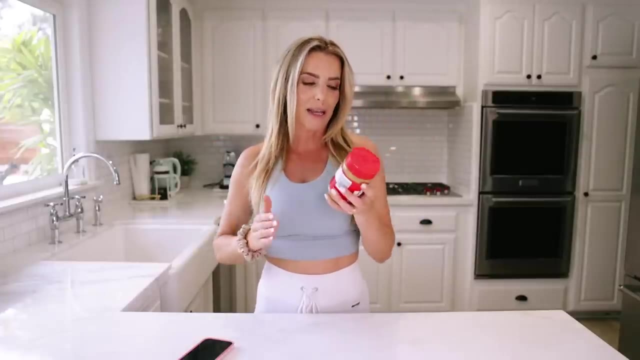 different brands. I'm confused. Um, okay, So this is just the standard peanut butter. It's creamy peanut butter. It shows you it's seven grams of protein, Like that's great per serving. So you got to go back and look at the label, though, So we know it has seven grams of protein, 16 grams of. 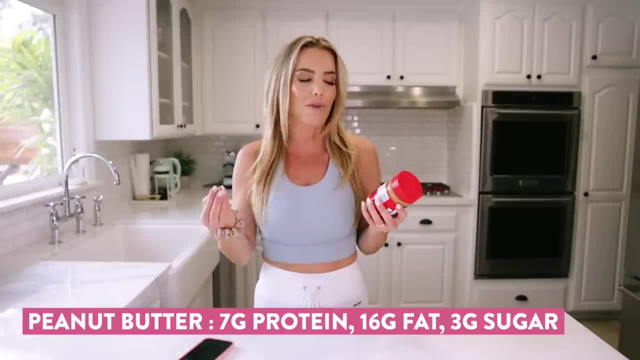 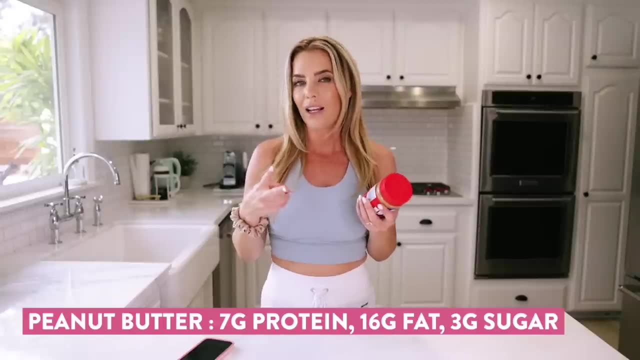 fat. That's fine, You guys. it's healthy fat. Peanuts are a great source of fat and protein- Awesome, Helps curb cravings- Cool. But it has three grams of sugar. Two of them are added, So they've added sugar. 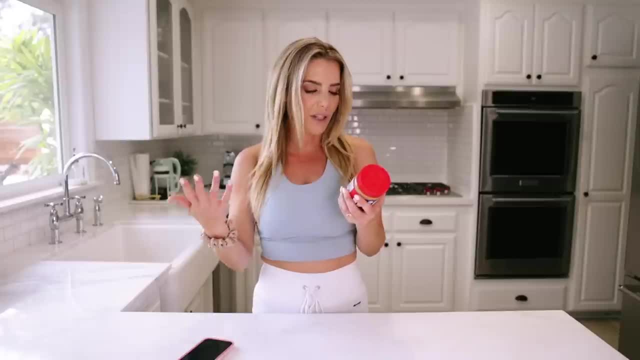 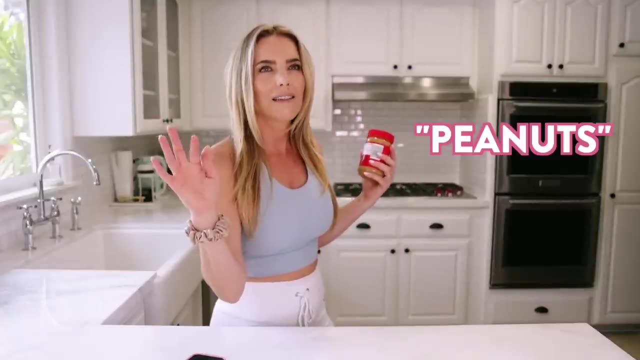 To this mix. Sodium is 6%. Like fine packaged foods are going to have that. protein, Like we said, is seven. So now I'm going to look at the ingredients. The ingredients should say peanuts, maybe a little salt, That's it. There shouldn't be anything else, but there is. So 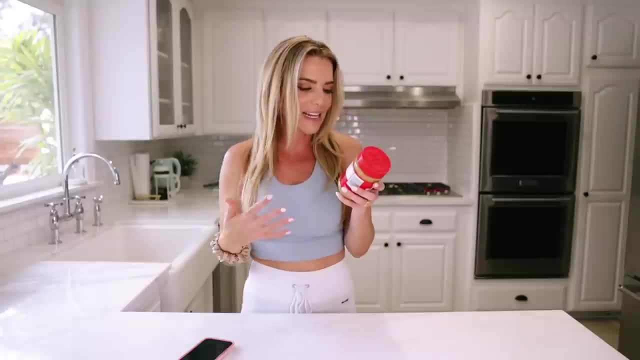 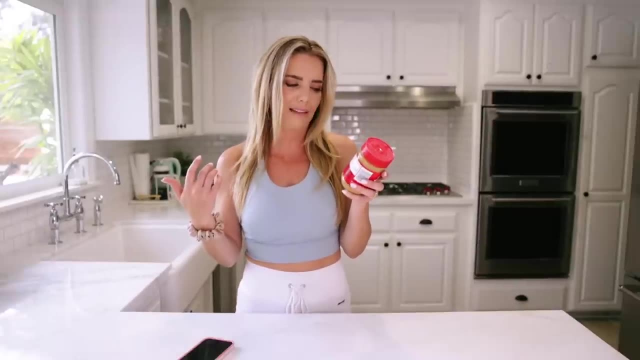 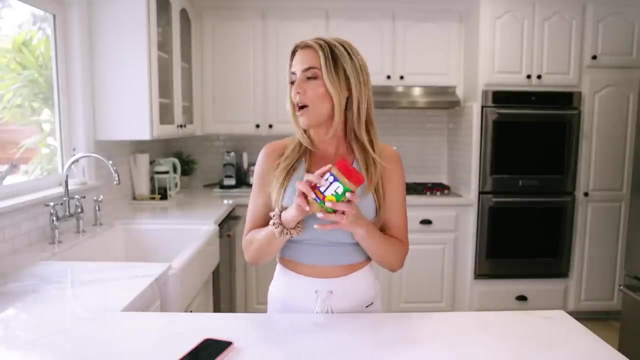 there's like roasted peanuts, sugar, molasses, fully hydrogenated grape seed- or it says, rapeseed- Is that a thing? And soybean oils- Um, and a bunch of other stuff like unnecessary, too many ingredients that you don't need to be putting in your body, So instead go for just a pure. 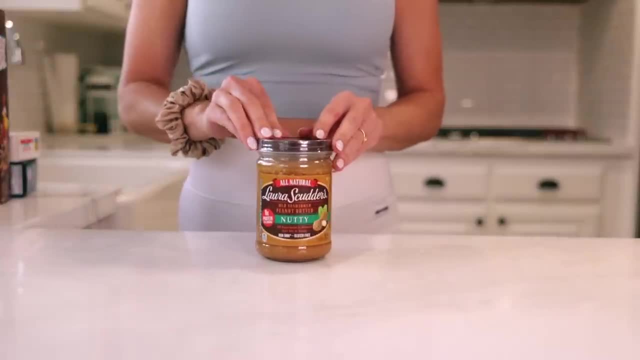 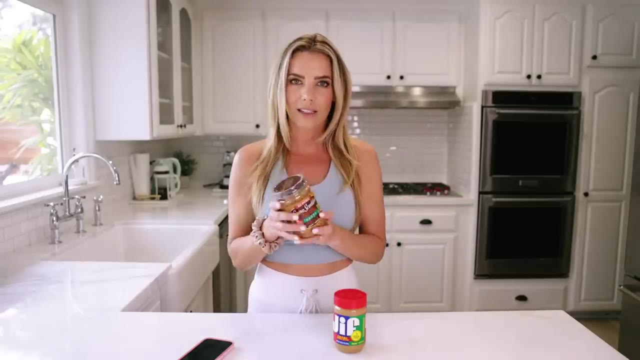 natural peanut butter. So this one is just old fashioned peanut butter. has eight grams of protein, Um, and it literally is peanuts and contains 1% or less of salt. That's it. So, like this is the ones you want to go for, just peanuts, maybe a little bit of salt, no added sugars, no added. 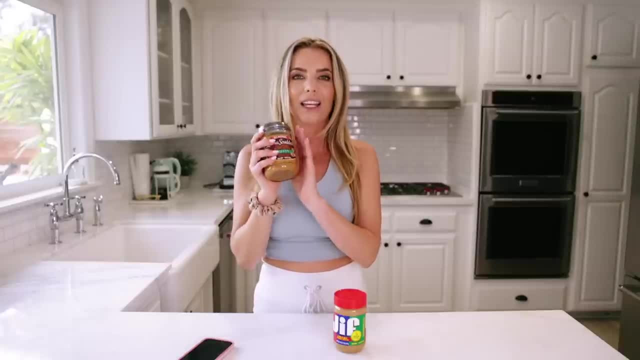 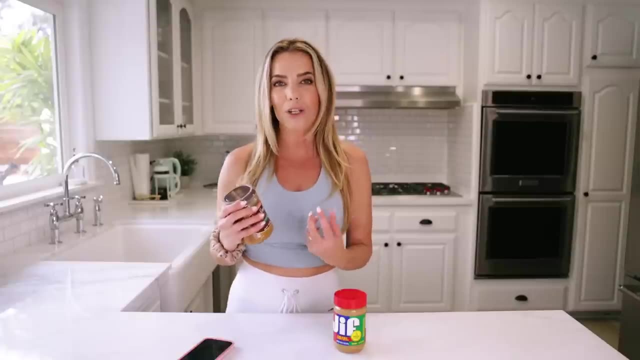 oils. Peanuts have a lot of natural oils, as is So like. just go for the real deal. It'll make a huge difference in the flavor. It'll be better tasting, It'll be better for you, You will stay full longer and you won't have all the added junk going into your body that you don't need. Where are my soda? 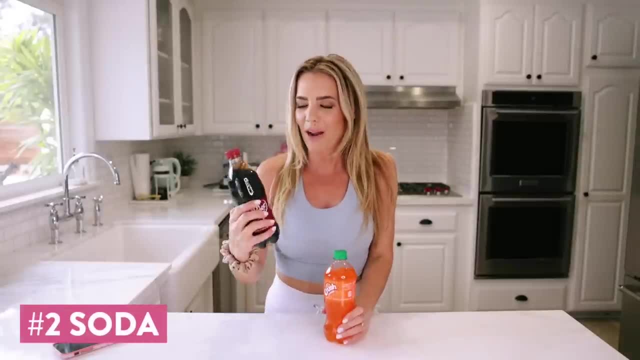 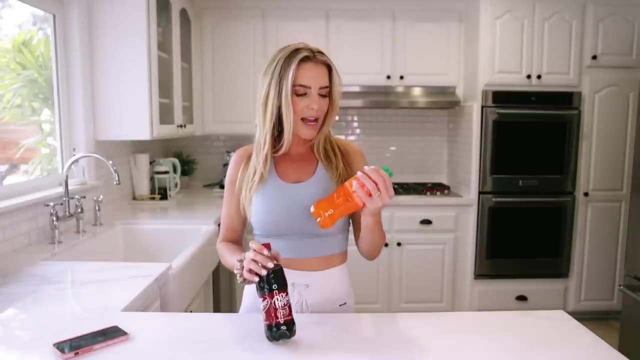 drinkers that I used to love Dr Pepper. I feel like you either love or hate Dr Pepper. I don't really know a lot of people that are like an in between indifferent. It's like a love hate thing. Um, okay, Got some orange crush, citrusy vibe Dr Pepper. It doesn't really matter what soda. 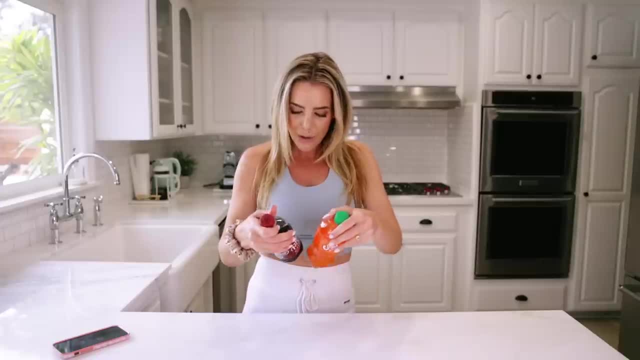 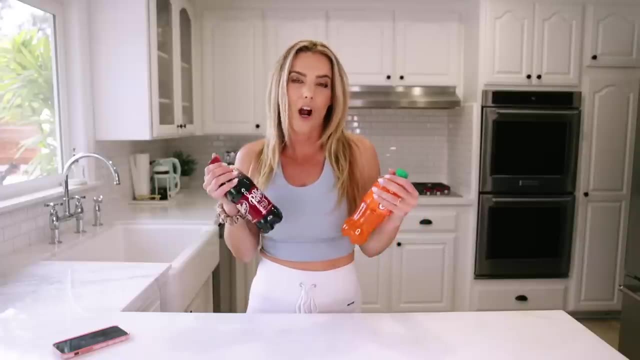 you're drinking. If you're drinking soda, you need to stop. Um, I don't know what the difference between these are as far as let's look at the what's in them: sugar wise Cause, literally that's all it is. It's basically carbonated, chemically sugary water. Yeah, Water. 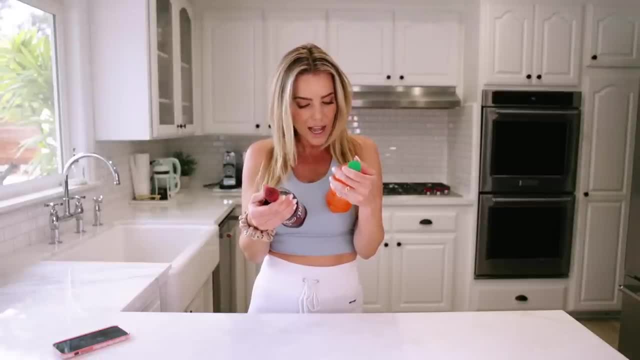 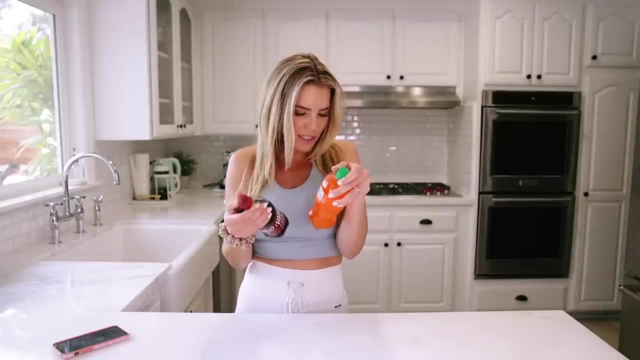 carbonated water, high fructose, corn syrup, citrus acid, um, all natural flavors, modified corn starch, some type of gum, yellow salt, all these dyes- I mean caramel, artificial flavors. Okay, But let's talk about the sugar. 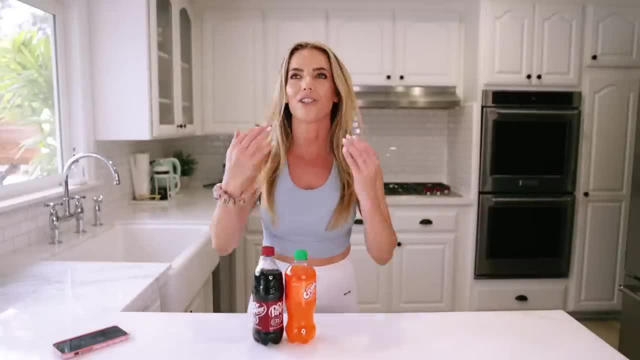 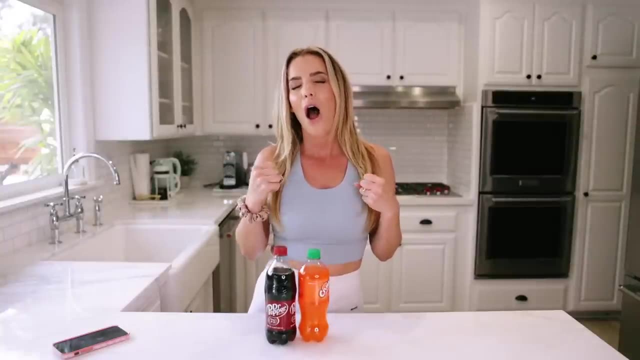 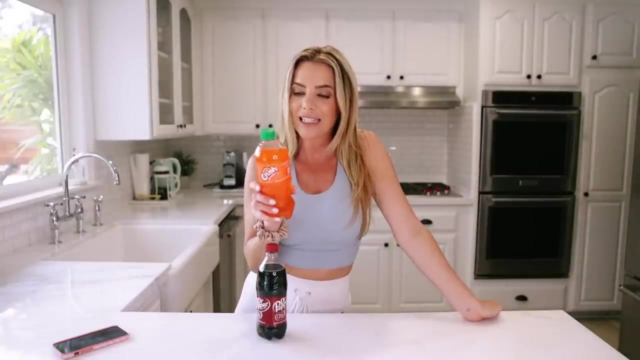 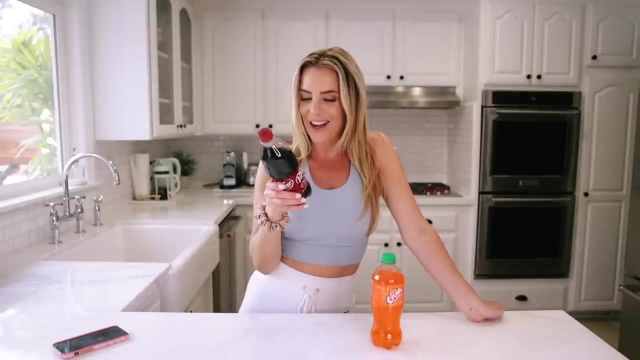 Literally, I can't. even So, when I was younger I used to drink like Cokes and Dr Pepper's and I'd get like the 32 ounce, sometimes the 44 ounce, and be like summer day. I can't believe it. now that I know what's in them, It's crazy. Um, okay, So your orange crush, 71 grams of added sugar and Dr Pepper? Oh good, It's only 65.. Oh my gosh. So in this one bottle you're 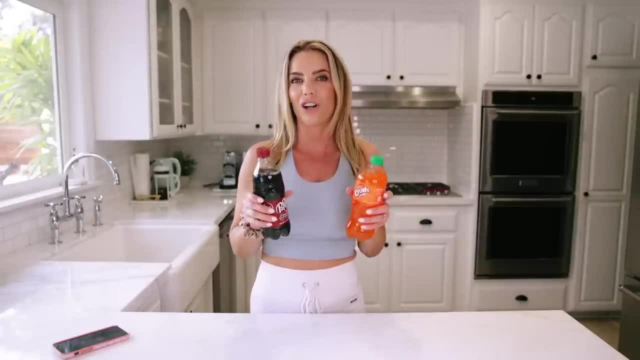 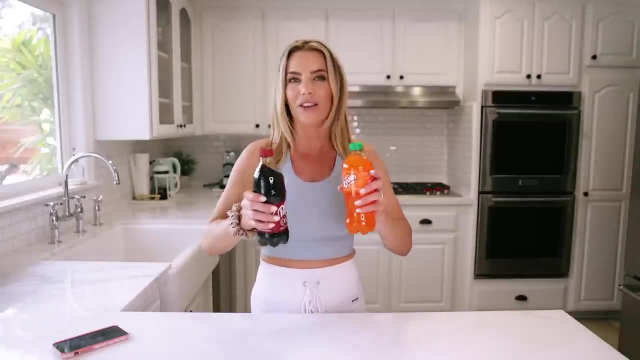 you're getting almost three times the amount of added sugar. that is really like recommended, allowed, okay in your day, in one and like no other benefits. There's nothing beneficial about this. I don't want to say other benefits. It's horrible, Like it's just horrible, There's nothing good. 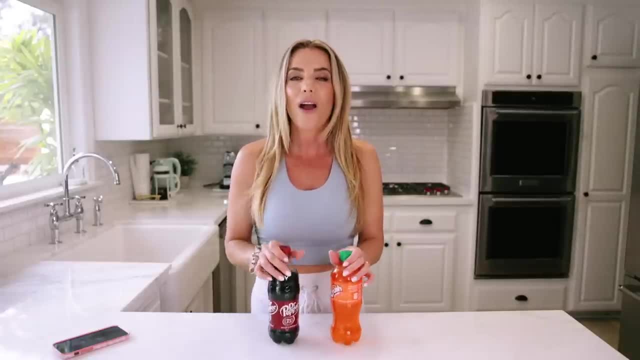 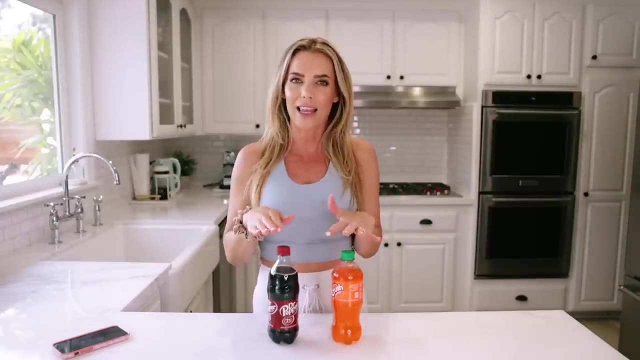 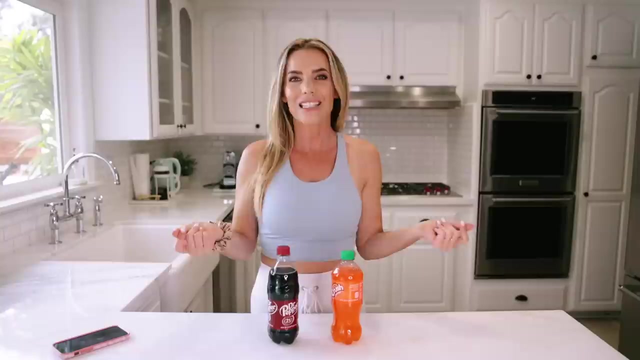 about it. You can argue with me till you're blue in the face. It's not okay. So if you are someone who likes that yummy kind of sweet carbonated drink, I get it Like I get wanting the carbonation, and I honestly also get that like just like flavored bubble. water doesn't always cut it and 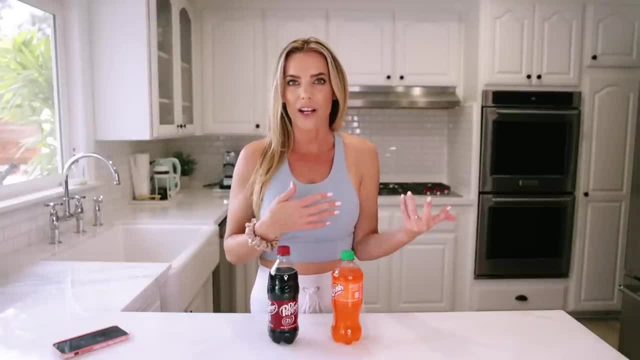 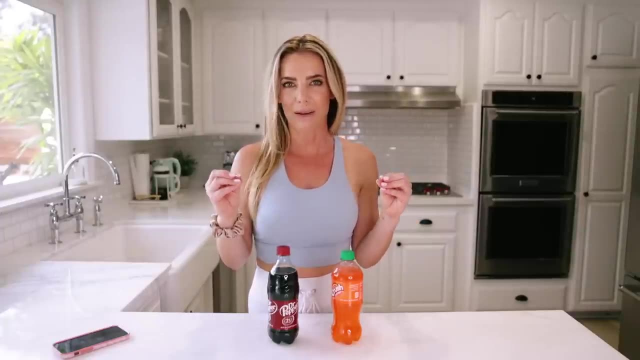 you don't really get any benefits from that either, right? So it might be sugar-free, so you're not getting the sugar, but you're just getting carbonated water. So here is my favorite hack. that is the best swap ever, and you are going to thank me for this one. So my swap for soda. 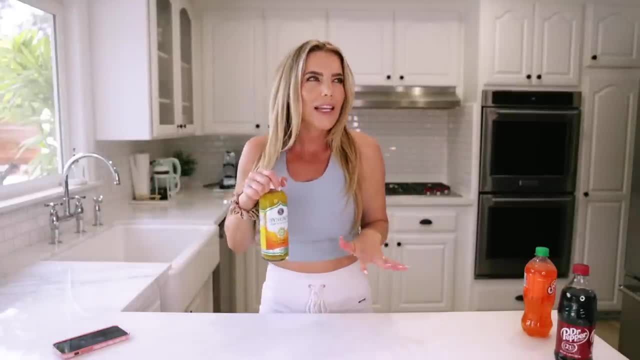 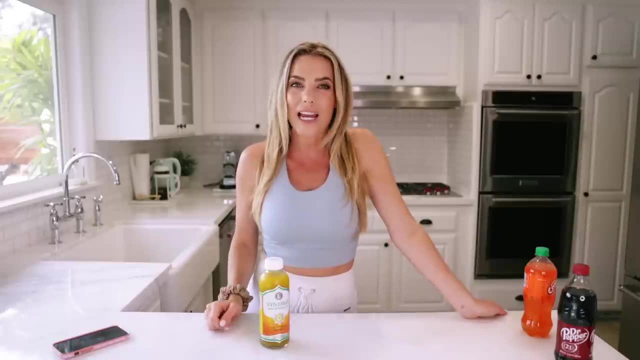 kombucha. If you guys haven't tried kombucha- or you're just like that's really hippy dippy- no, You have to try the GT Synergy. I've been drinking GTs for, honestly, probably almost 10 years, which is so crazy to think about. It is the first brand I ever had. I fell in love with. 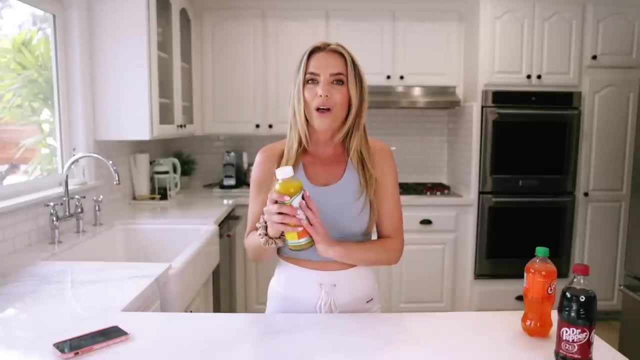 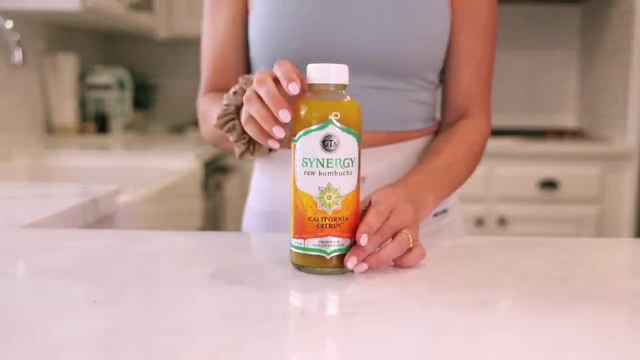 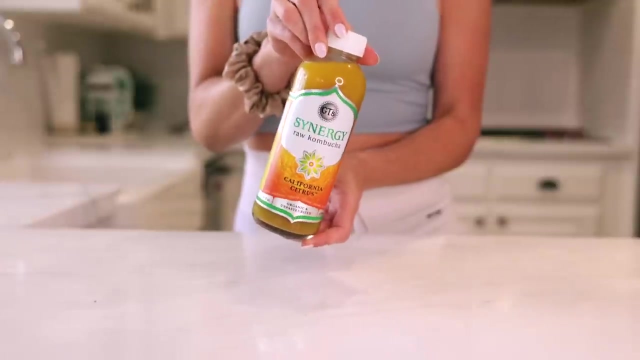 I've tried other ones. They're not the same. They're just not The quality, the taste, the flavor, the like. all of the different flavors they have are the best, Especially this flavor. If you guys are like more of like a citrusy orange crush soda drinker, the California citrus is so yummy It is. 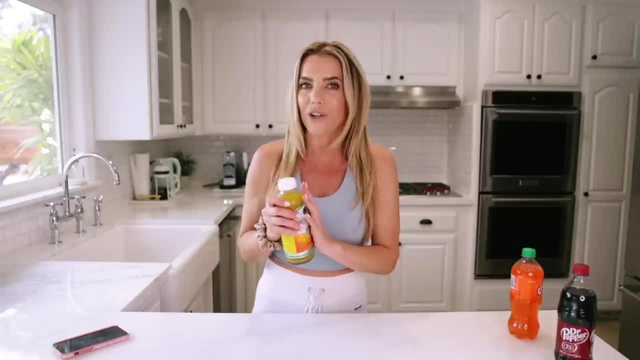 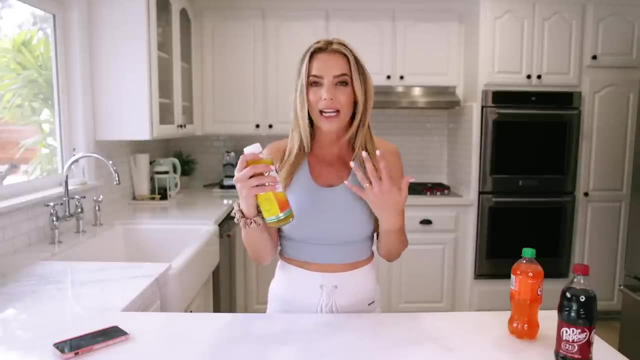 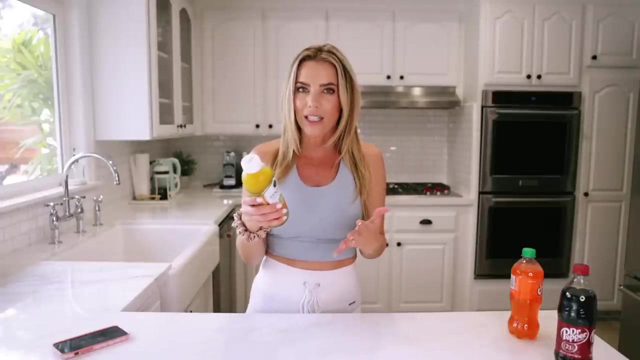 like packed with flavor, but it's also packed with nutrients. So you're not getting just bubbly sugar. it's bubbly, which is nice. You have that like almost carbonated feel from the kombucha, but it's organic, It's unpasteurized, It has so many incredible enzymes and probiotics for you. 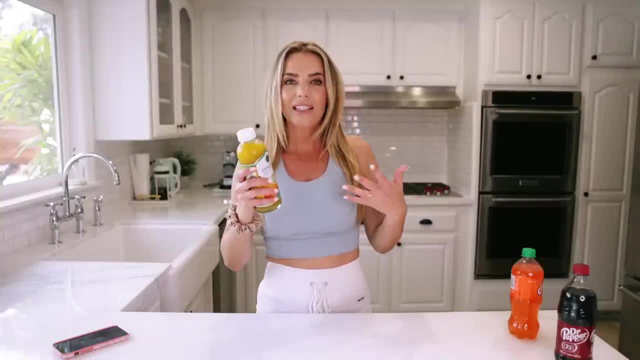 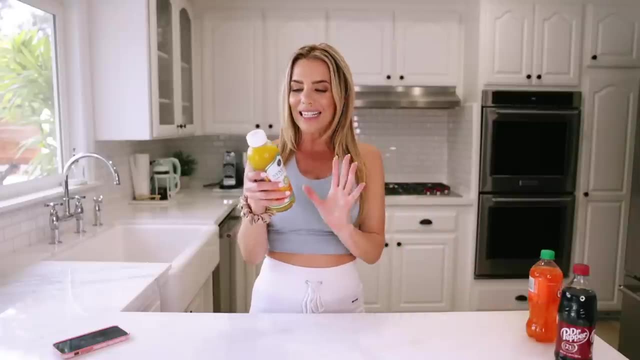 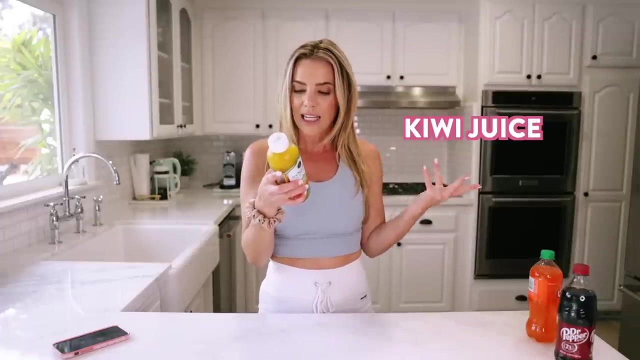 It only has 16 grams of sugar, which again is like you know, when you're looking at different things. We just talked about this one. This has 71 grams of sugar. What So? only 16, and it's from good stuff. So ingredients: in here you have GTs, kombucha, black tea, green tea, kiwi juice. 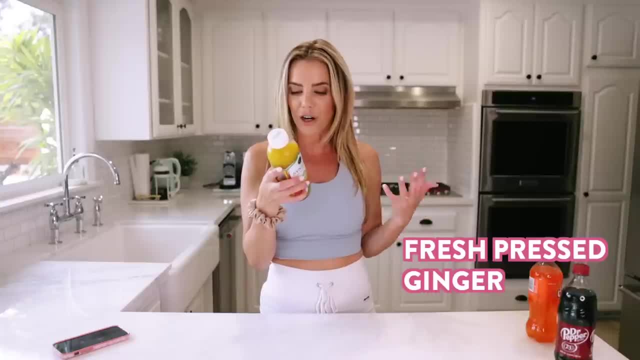 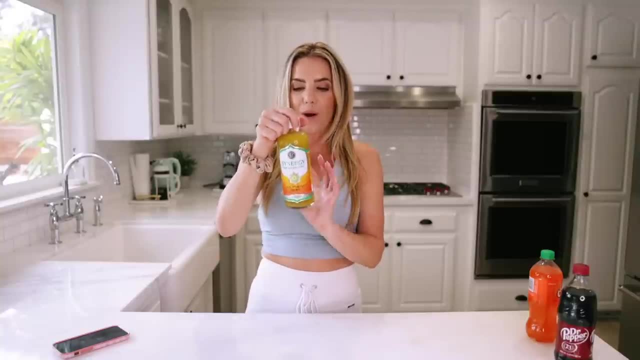 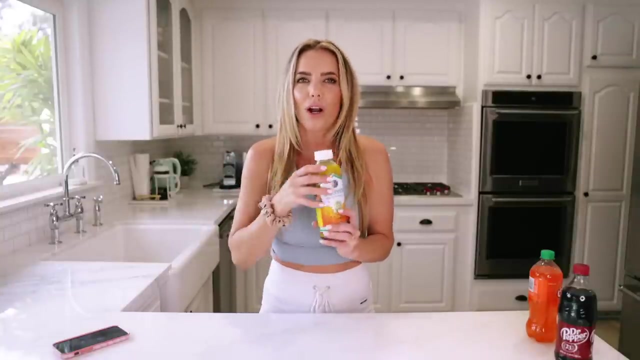 kumquat, puree Meyer lemon, apricot fresh, fresh ginger, vanilla extract and 100% pure love. So the sugar you're getting is from real foods, real things like right in here It is. I don't even like, I don't even know what to say. It's just like the best swap you could ever ask for for a soda. 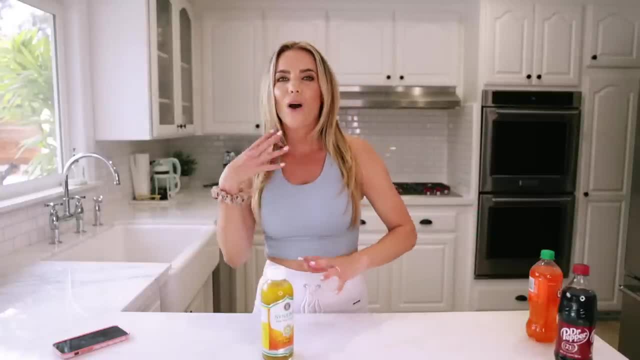 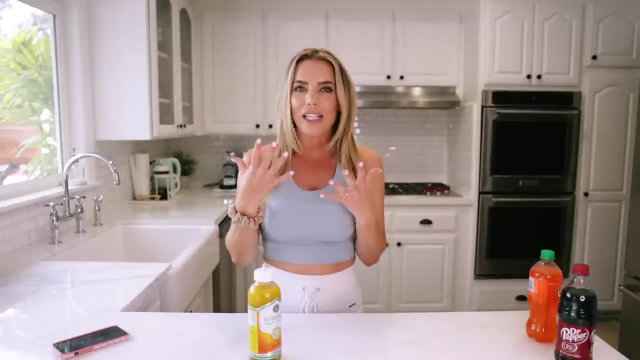 They have tons of different ones, like I love their gingerade. They have, like watermelon, So many different flavors. So if you are someone who likes to mix things up, if you need to have that flavorful drink every day, you need to try kombuchas, And I'll put a link down below for GT Synergy, so you 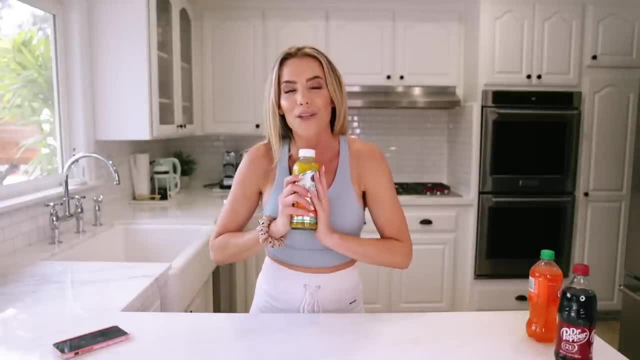 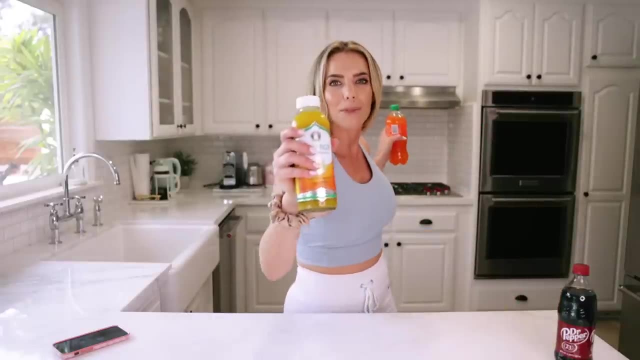 guys can go to their website and like see all the stuff they have, because they're amazing. I love partnering with them And if you guys are doing summer shape up, you can also win a year's supply of GTs, which will just get you all set up to make your swap super easy. I don't know about you guys. 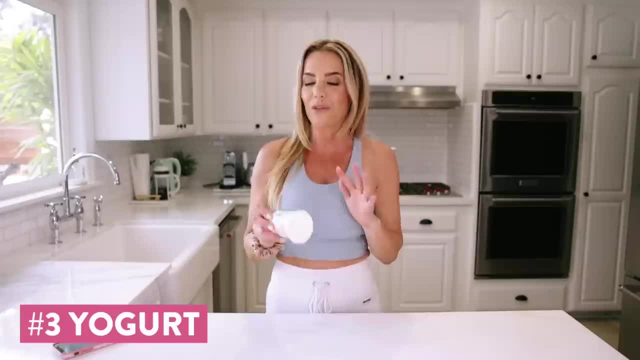 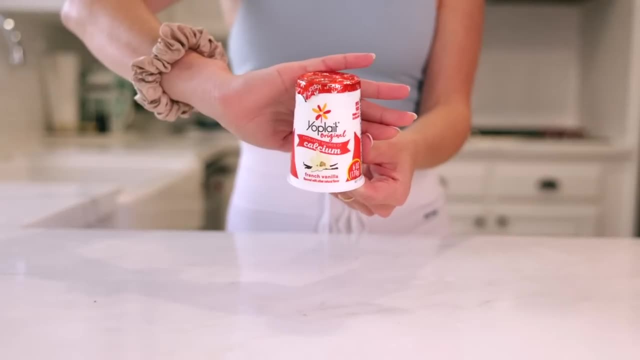 but I used to eat yogurt for breakfast every single morning and I would do it for dessert all the time. I just was like it's a healthy snack. So this is just like a Yoplait original, excellent source of calcium, Cool. So this is one of the brands I used to have all the time And if you look at the back, 150 calories. 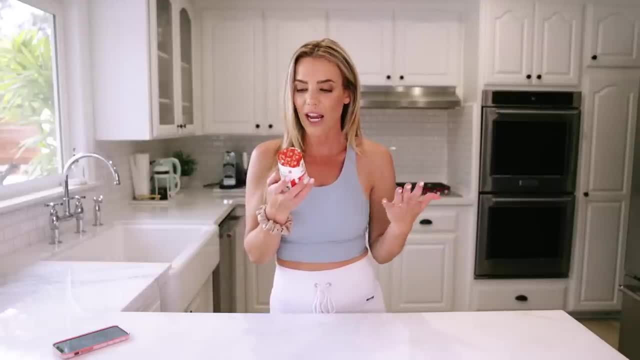 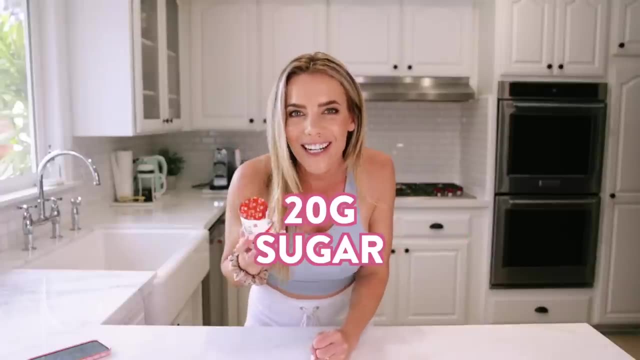 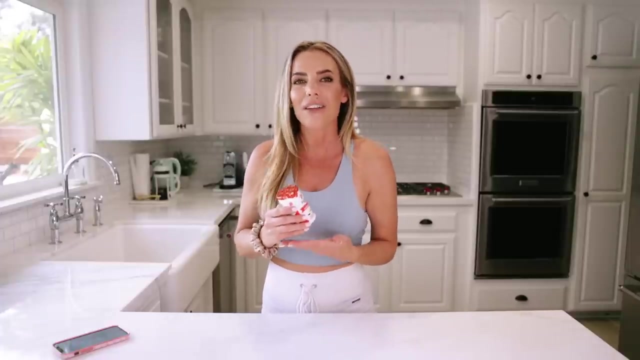 cool, That's not bad. Like you're gonna have this with some cereal or something Great. Only two grams of fat, That sounds nice. 28 carbs, 20 grams of sugar. Oh my gosh, you guys. it's so tiny, So really we're only supposed to be having like 24 grams of added. 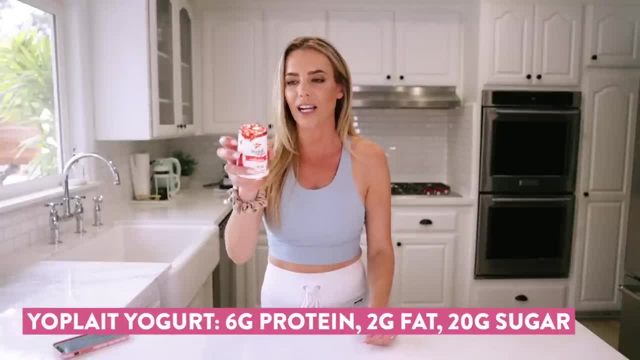 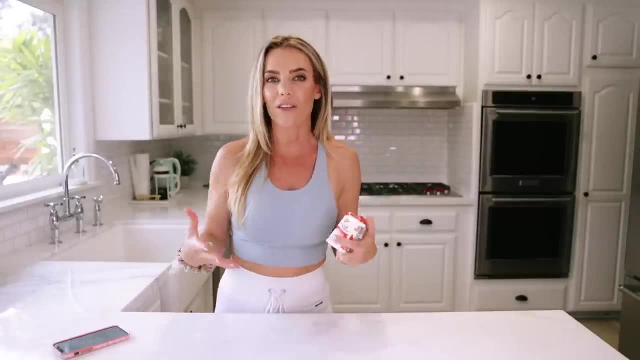 sugar every single day in our diets, you guys? I think here's 20 right here And it has six grams of protein. So, like, fine, whatever, A better choice if you are a yogurt lover, like I love yogurt And I usually. 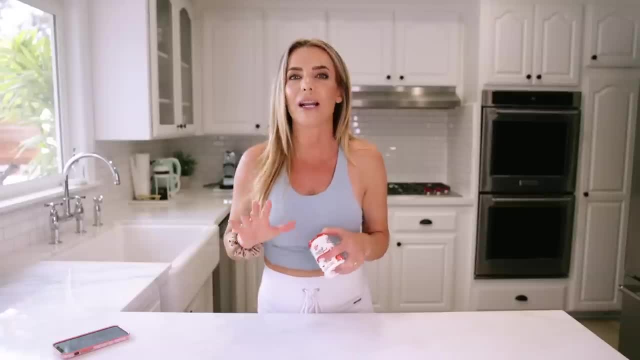 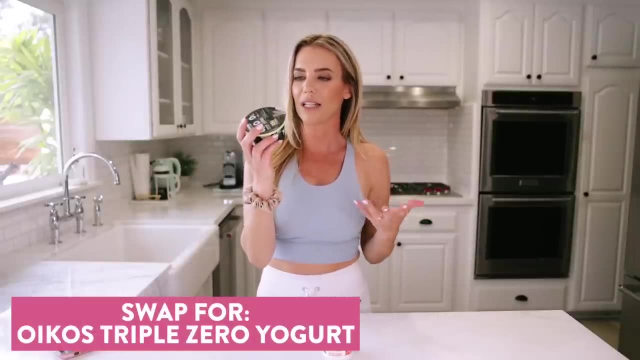 will do like plain Greek yogurt, So I don't get any of the sugars and stuff. But I know that that's like not ideal for a lot of people, But something like this is a great option. So this is a triple zero. It has 15 grams of protein, zero grams of added sugar. It's only 100 calories. you actually 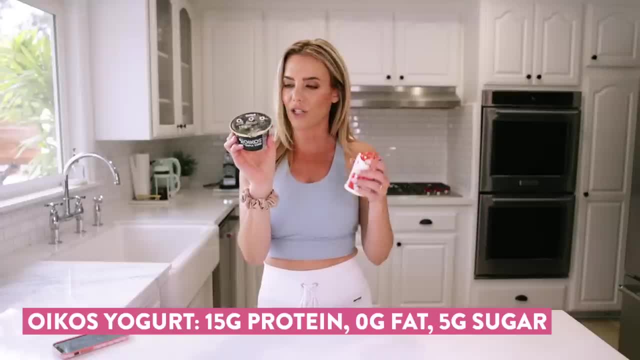 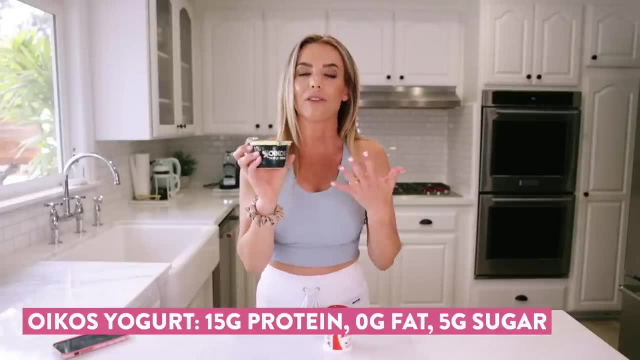 are getting less calories. You have zero grams of fat, where this one has two and 15 grams of protein, When this only has six. And then again this one has no added sugar. it has five grams of sugar in it, But that's natural from the milk like that you use that makes yogurt. That's just natural. 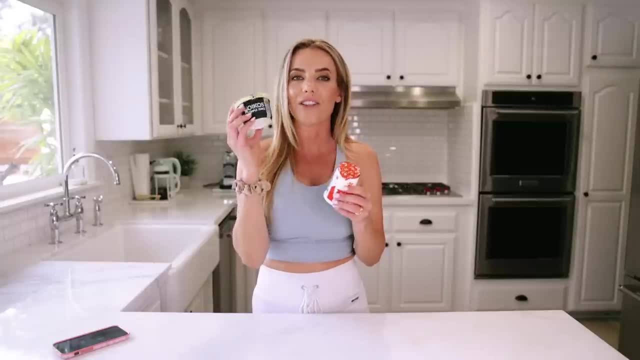 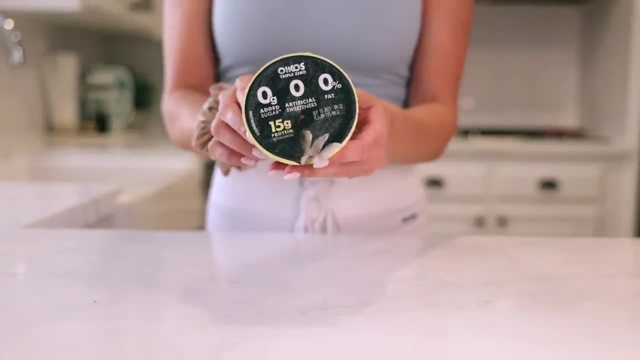 So only five grams and you're getting 15 grams of protein And it's still that vanilla flavor. So vanilla, vanilla, it has a taste, It's yummy. It's not going to be like plain and sour or anything. If you are a yogurt person, make the swap Again. 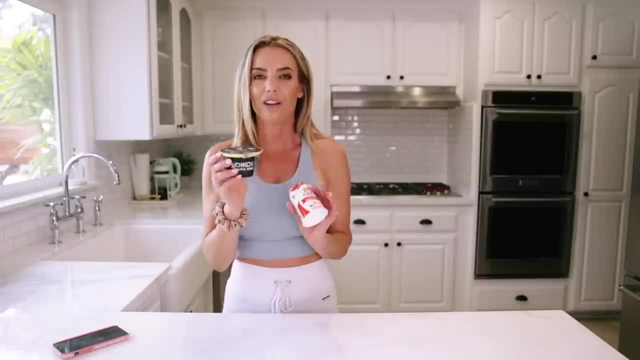 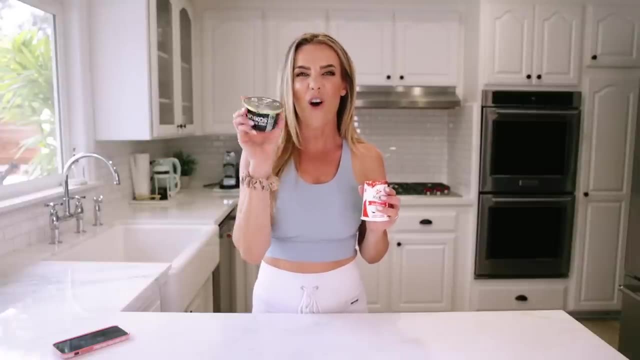 I always like to try to stick to something like under five grams of sugar, five or under. So this is good. And again, it's not added sugar, It's just the real deal already in it from the milk and you get all that protein to moving on to cereal. So last video I talked about how I used 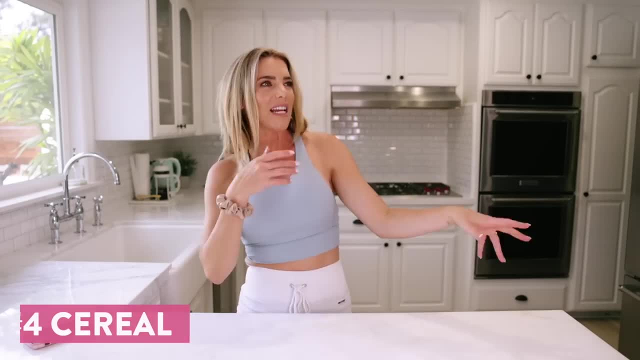 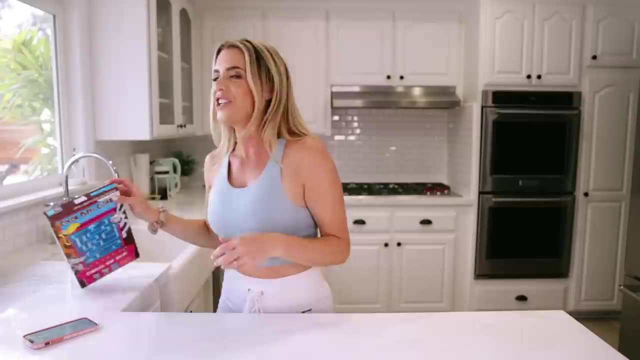 to eat this one cereal. I'll just tell you a special K that it was like eat two a day and you're gonna lose all this weight, And I swapped it for protein pancakes, which are a way better choice. But if you are someone who loves cereal and you're like: don't give me all the sugar cereal. 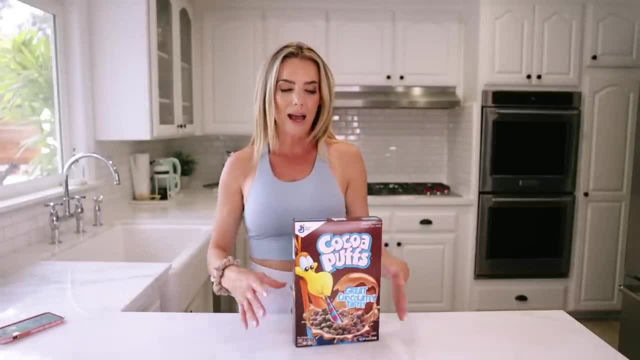 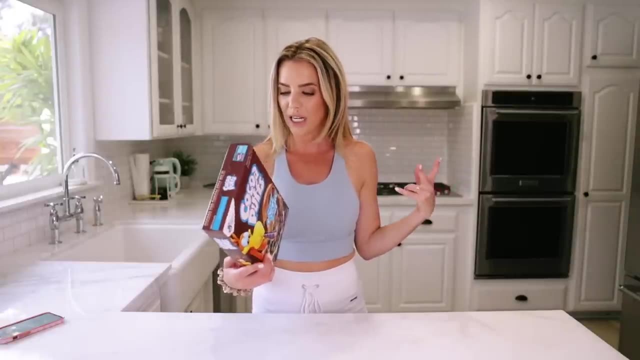 I wanted to give you guys a better for you cereal swap Because, like Cocoa Puffs, right, we have. how much sugar? 12 grams. I've added sugar. only two grams of protein. the ingredients, as you can imagine: whole grain corn. 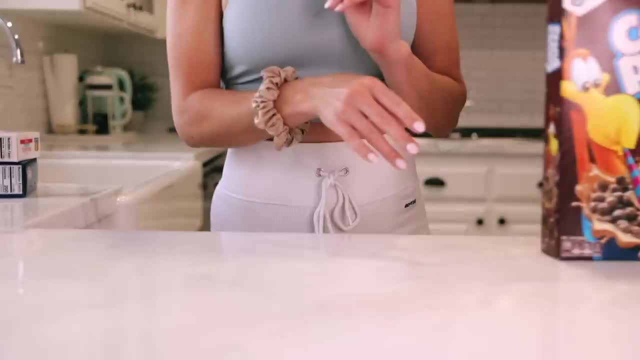 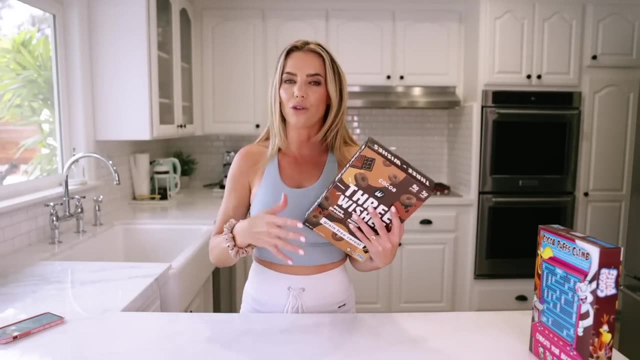 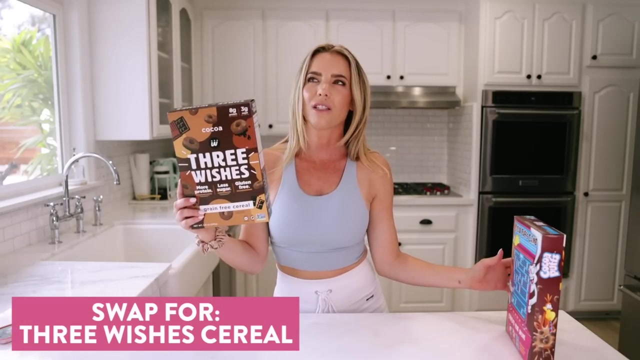 sugar, rice flour, corn syrup, cocoa, blah, blah, blah, blah, blah. tons of just like no ingredients. So there are a lot of brands now doing more like protein, low sugar, healthy, better for you, cereal swap. So this one was good because it was Cocoa Cocoa. This is three wishes. 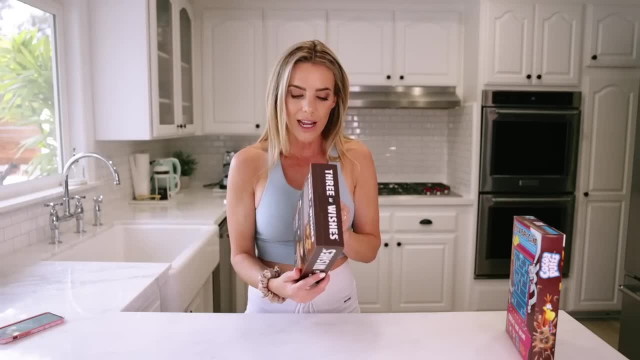 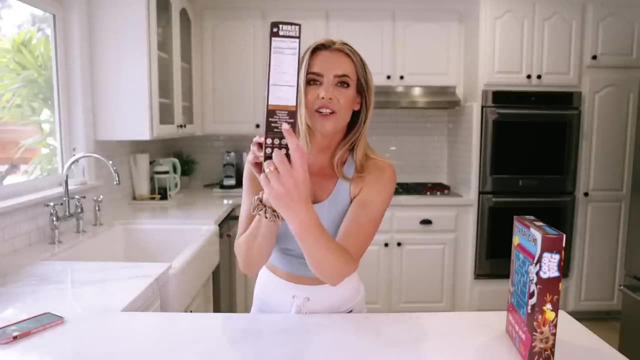 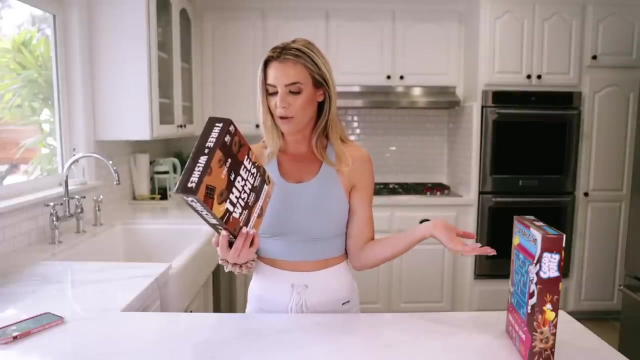 There's another one magic spoon that I really love, But if you look at, it has eight grams of protein but only has three grams of sugar, which is like nothing. And you can see their ingredients right there: chickpea, tapioca, pea protein, organic cane, sugar, cocoa, natural flavor, salt and monk fruit. 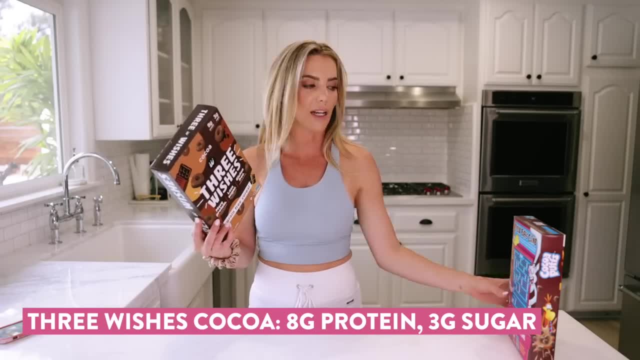 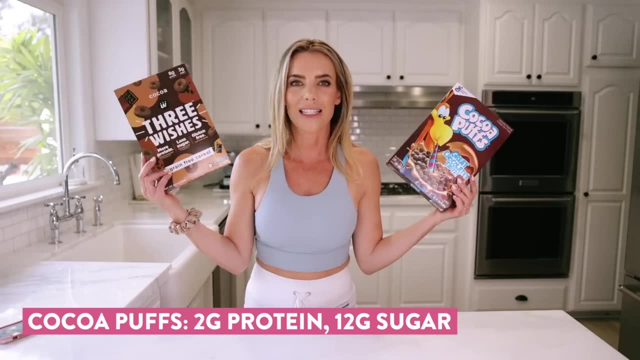 simple, clean. you're getting eight grams of protein per serving, compared to what was this one to, which is nothing. And then this one is 12 grams of sugar. This only has three. it's an easy, obvious swap. So if you still have your Cocoa Puffs, swap it for this. I love a good. pasta. I love it. It's really good. It's one of those things it's really good And then if you're like I don't know what to do with it, I'll make another one And I'm going to skip them If you're. 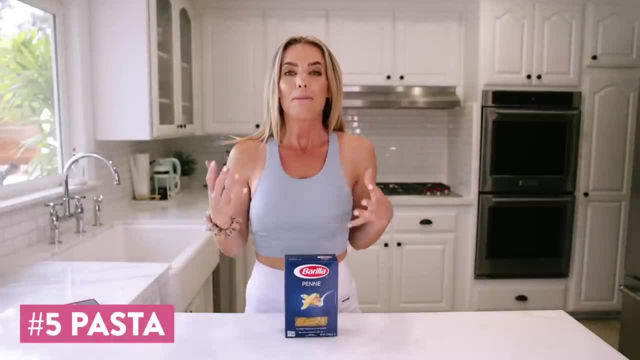 like I don't know what to do with it. I'm going to make another one If you're like I don't know what to do with it. I love Italian food- like, give me all the pasta, but, as you can imagine, it's not always the healthiest. 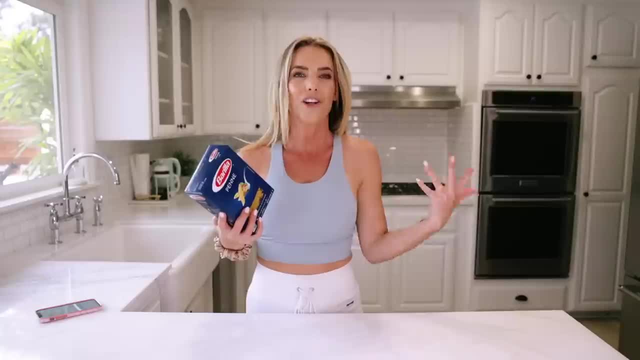 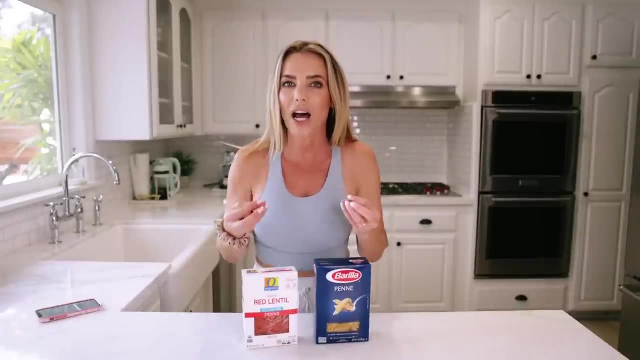 thing and it's really just the way that it's processed. the flours that are used like you're not getting a lot out of your pasta. so I found a really good swap that I like to use and it's like a real pasta feel. I'm not just talking about swap it for spaghetti squash or zoodles, of course you. 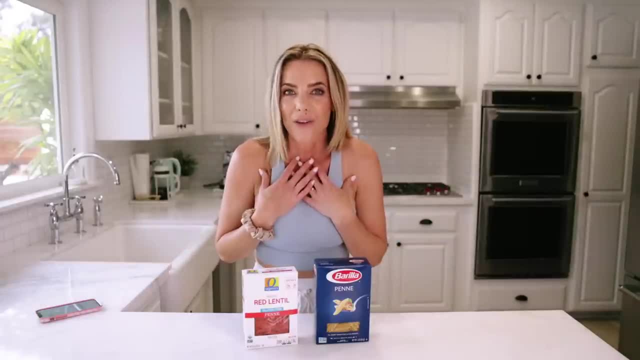 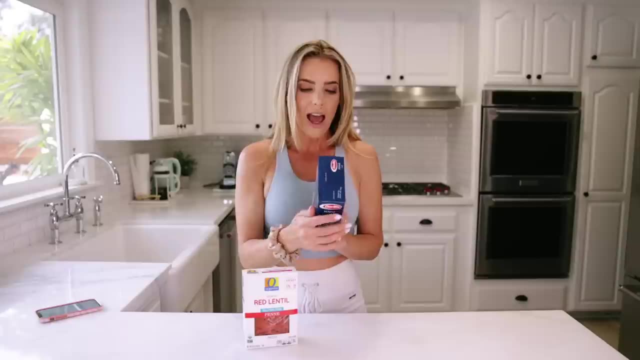 can do that if you're trying to be super, super healthy, and those are great. I love those things. however, sometimes you just want pasta. so this one that's just like your traditional penne. um, it has seven grams of protein, just like fair. like only one gram of sugar, one gram of fat, whatever. 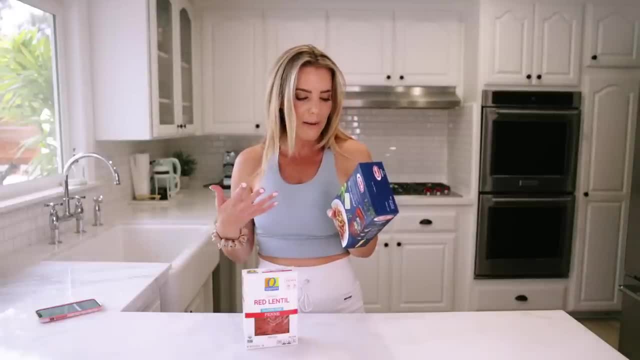 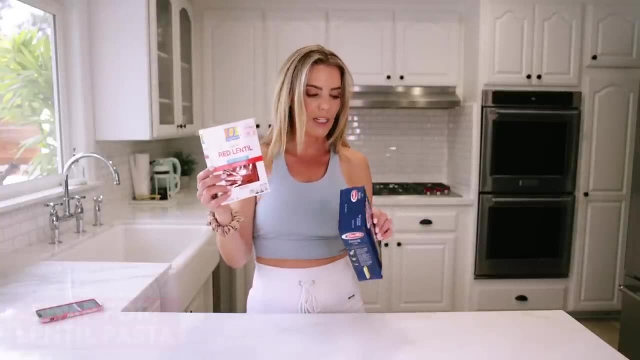 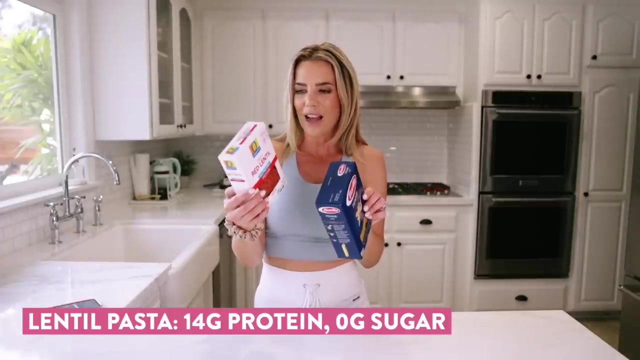 um, but it's just like different types of- like bleached wheat flours versus this red lentil pasta. this has 14 grams of protein, so seven per serving. same serving size: 14, so you're getting double the protein. um, everything else is pretty much the same, except that this is made with red lentil flour instead of 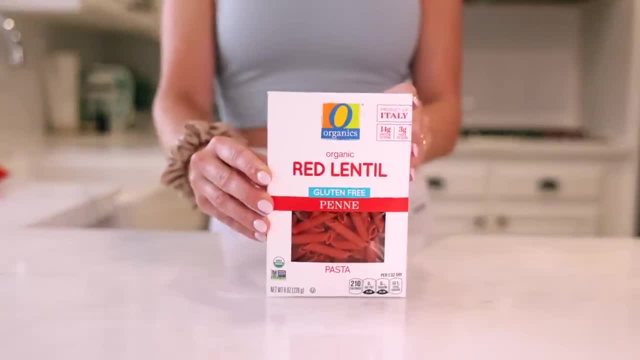 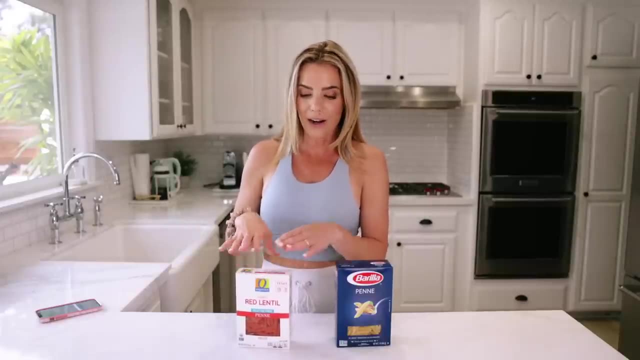 wheat flour. so also if you have a gluten intolerance, this is a better option. but this is one of those things that's really just about the quality of what you're putting in your body. red lentil flour is obviously going to be a lot better and then getting more out of it. so if you're gonna 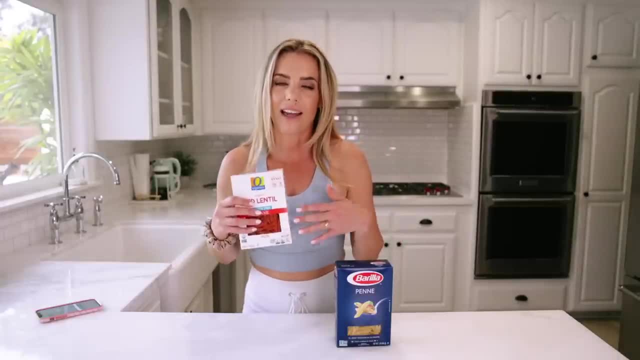 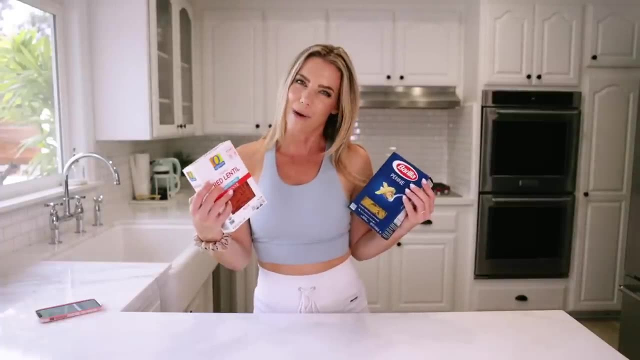 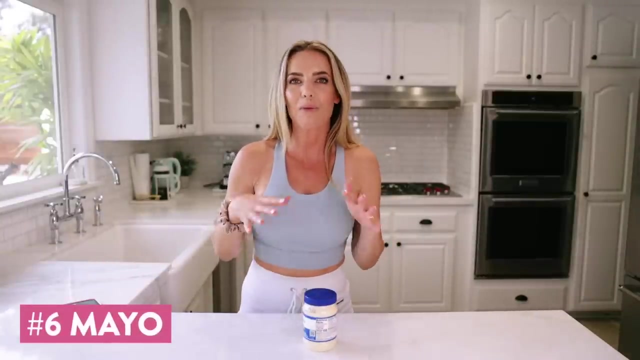 eat it. if you're gonna get the pasta, then get more protein, get that benefit from it. just comparing those things, something like this red lentil one would be a much better choice to still get your pasta fix. okay, number seven swap is a mayonnaise swap, and i putting this here because i feel like most people 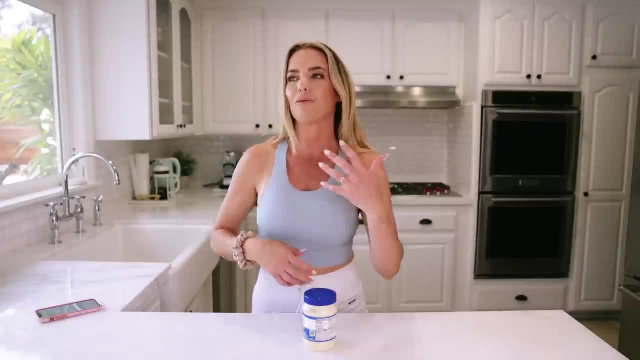 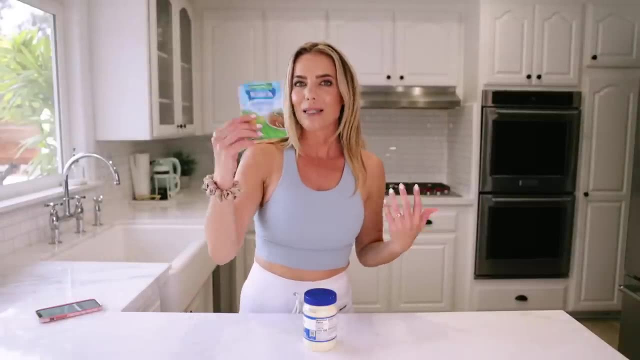 like to use mayonnaise in some way. like you're putting on a sandwich, you're mixing like egg salad, you're making a dip like a ranch dip. the ranch dip itself is not bad. it's a bunch of seasoning. maybe it has like high salt, whatever. but in general, like this isn't the problem, it's. 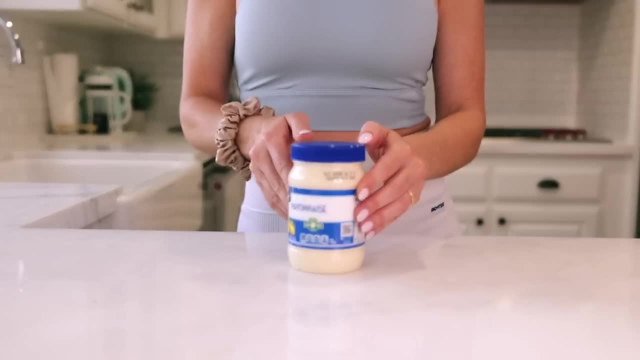 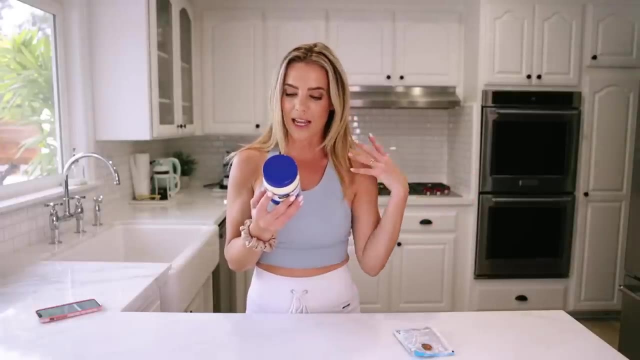 what you're putting it into. that's the problem. so this is just like a store-brand mayonnaise. there's no protein, 11 grams of fat, obviously, but the ingredients you're going to use on and off the edges are like a lot of different kinds of mayonnaise. 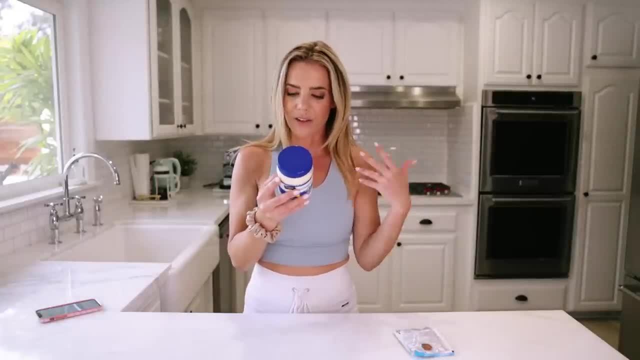 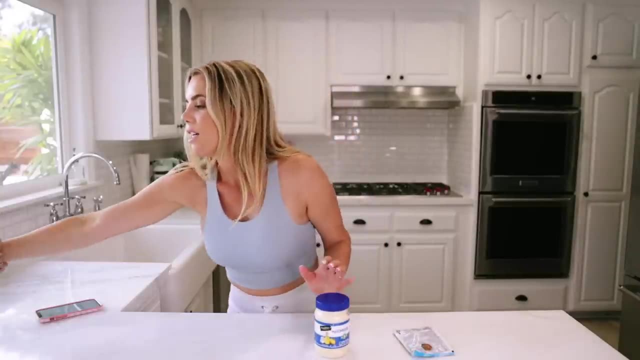 it's not going to be an easy thing to use, but this is where i started to have a problem, because it's like the first ingredients- soybean oil, water- then there's eggs, then there's sugars and lemon juice and natural flavors and artificial flavors and all sorts of craziness again, this is one of those. 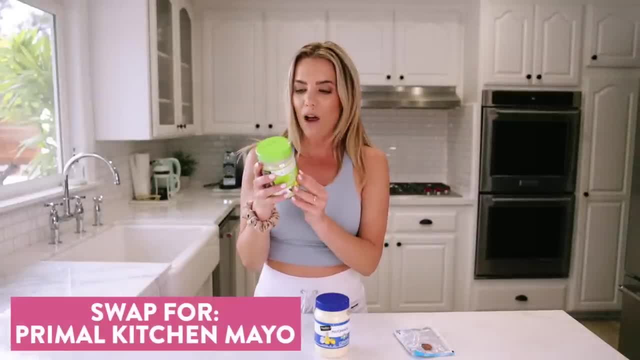 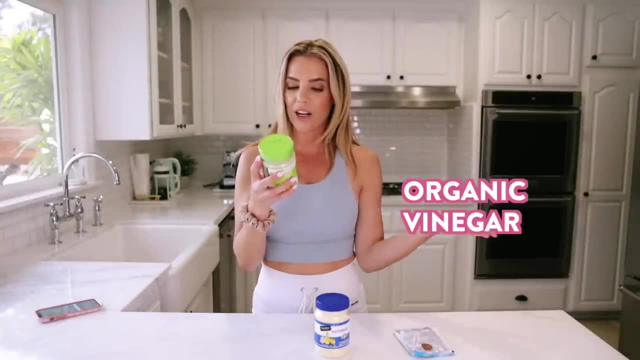 foods that should be very simple and very clean. so my swap for a mayo- if i still want that like tart mayo feel- is just real mayo. it's made with avocado oil. the ingredients are literally just avocado oil, organic eggs, organic egg yolk, organic vinegar, sea salt and mandarin. actually its a pretty with a pick. 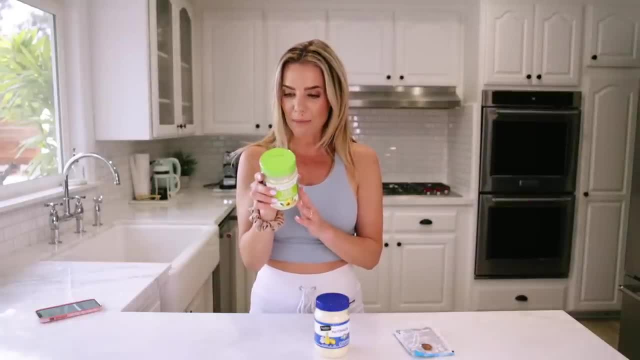 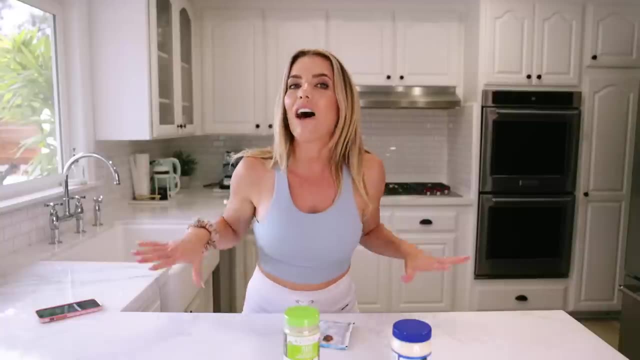 rosemary. that's it. super clean, super simple. so if you're going to make your dip, go with something like this primal kitchen mayo that is made with the avocado. and if you want to be even healthier, if you want to lose extra weight, if you're trying to be more strict on your calories, 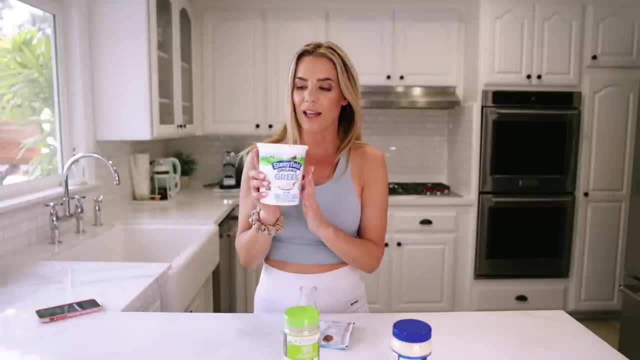 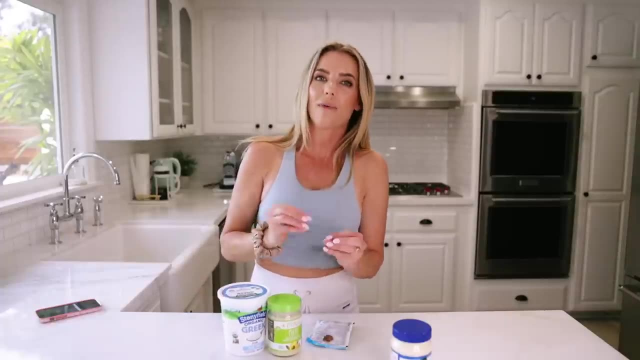 then a better thing to do is swap it for something like the zero percent greek yogurt or split the difference. do half and half, then i'm getting way more benefits: more protein, a little bit less calories, less of the fat in a dip because i'm just dipping it snacking. it's not like. 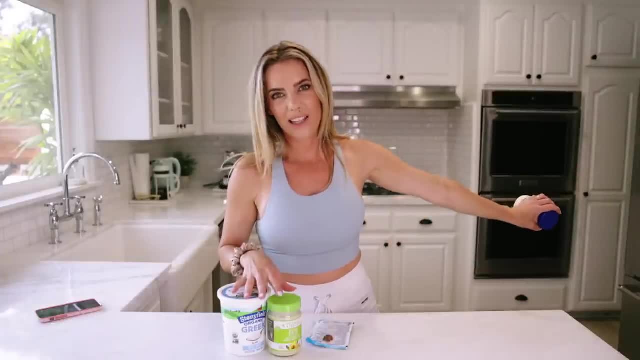 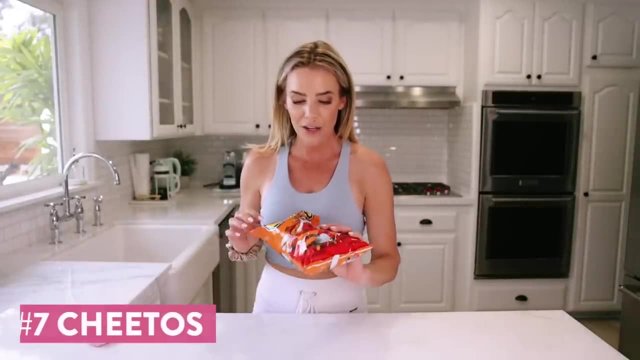 my main food source and i get rid of all the junk from one of these cheetos. i in high school, went through this phase where i ate flaming cheetos. these are regular ones. i didn't get the flaming ones because i was like i don't want to go there, but i used to eat the. 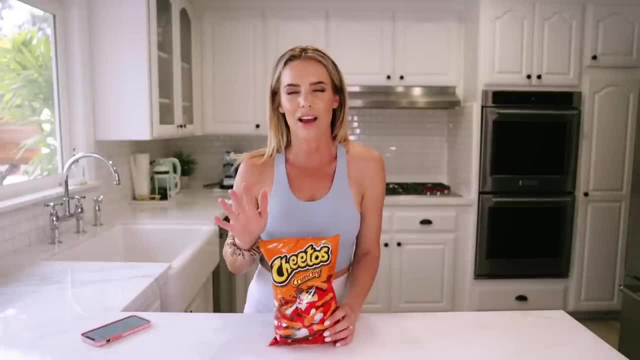 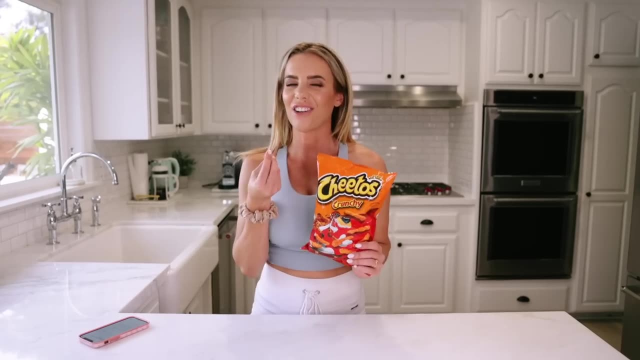 flaming ones like non-stop for lunch, like it was not a healthy diet, obviously for a lot of reasons, but i would like have that be like my lunch often. um, i get it- cheetos. they get on your fingers. it's all like yummy and delicious and cheesy and orange and whatever. but 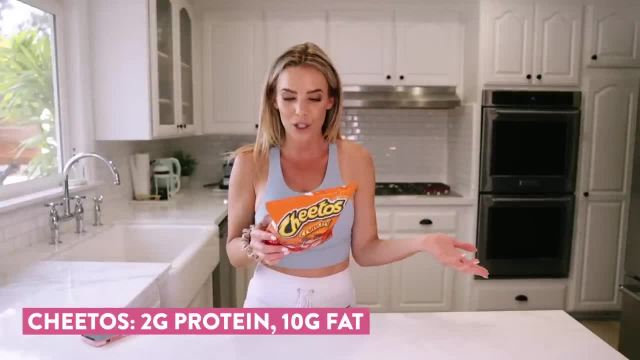 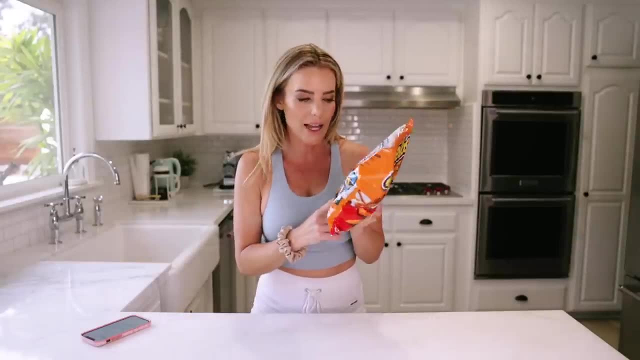 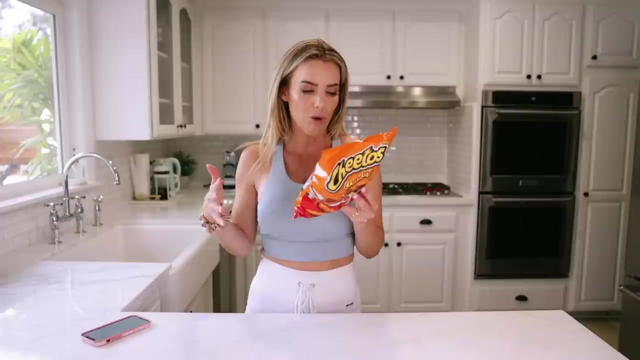 again 10 grams of fat. fine proteins- only two, like we know. we know this is like an extra snack, but when you go into like the ingredients again, it's a long long list, first one being enriched corn meal with a bunch of words that i literally can't pronounce. after it, vegetable oils with a million. 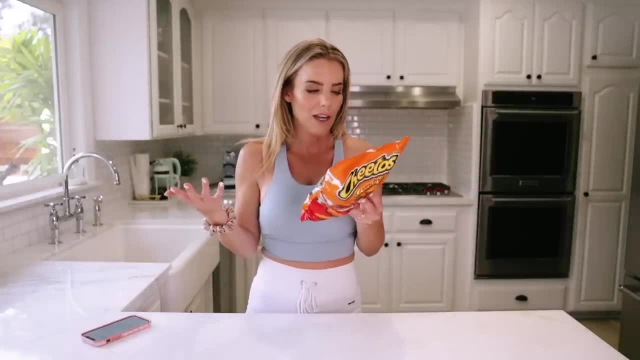 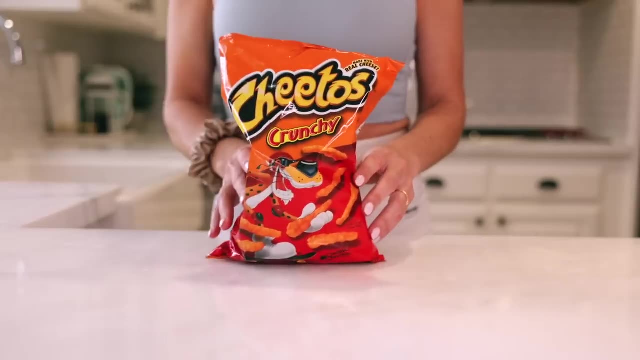 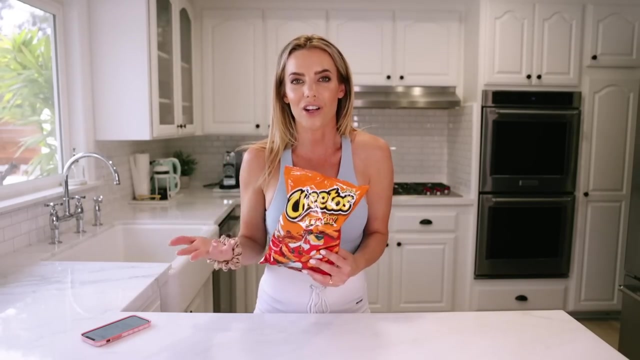 options of those. some cheese seasoning, like. what does that mean? um, natural and artificial flavors. like you, you get the idea. it's a laundry list of very overly processed foods that will impact our bodies over time. so if you're doing this like as a snack one, obviously you're getting a lot of extra calories. 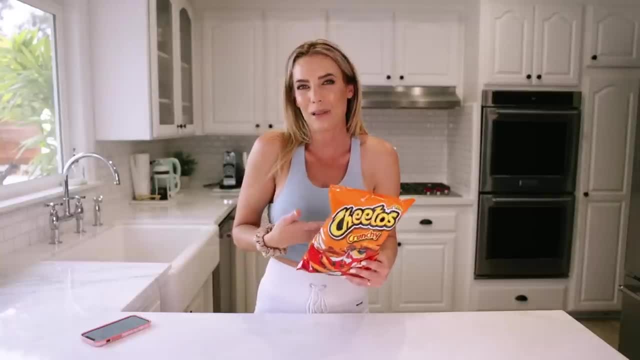 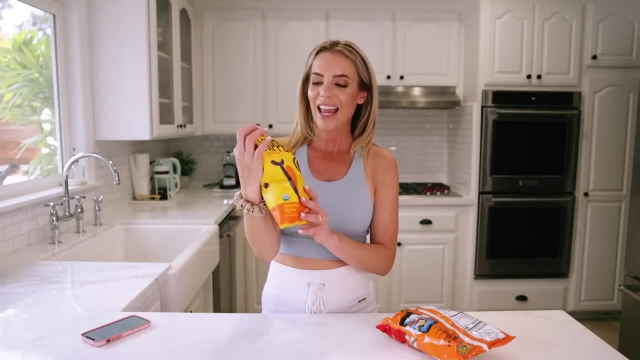 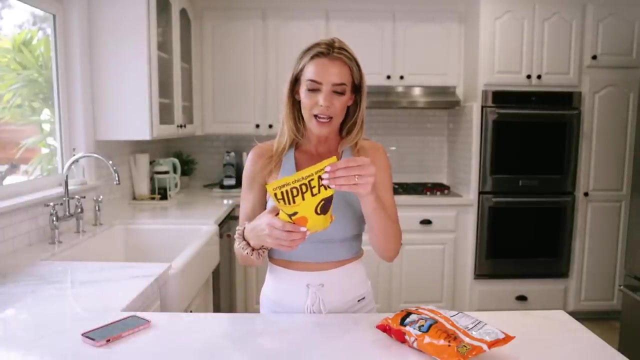 you don't need, but you're also getting a lot of like chemically processed foods that you don't need either. so healthier swap to still get your cheeto fix is these hippies. there's other brands that do a similar thing, but they're made with organic chickpea, like flour, basically. so if you're 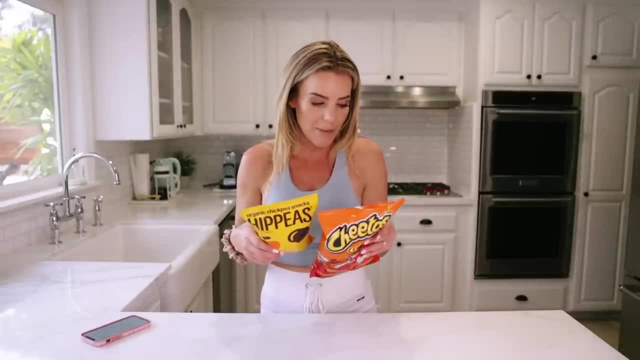 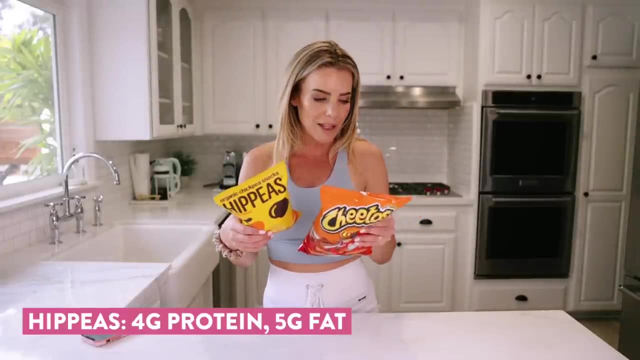 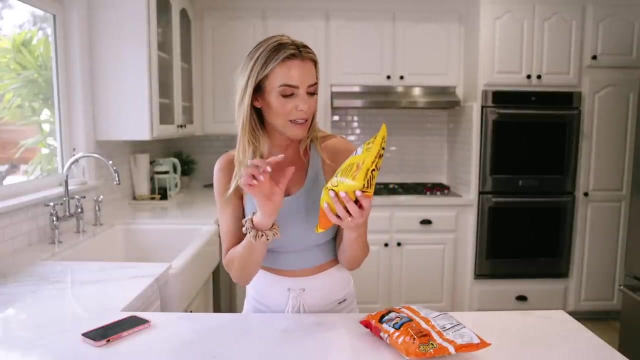 just looking like. serving size is about the same. so in the same serving you get 10 grams of fat. you only have five grams of fat. um, in this one you only have two grams of protein. you get four grams of protein. and the ingredient list is clean, baby simple. there's like maybe six or seven things. 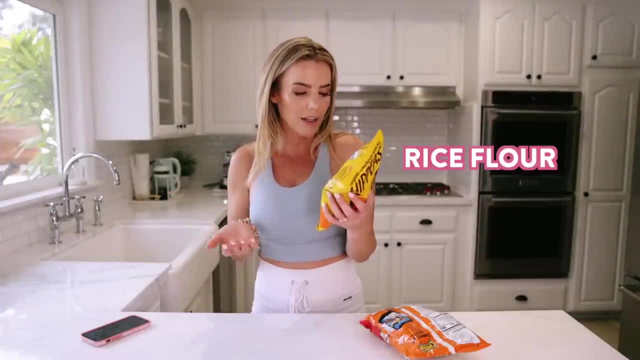 organic yeast, chickpea flour, organic rice flour, sunflower oil, tapioca starch fiber. it's just such a better option for you. so if you're looking for something that's going to help you with your weight loss, and you're looking for something that's going to help you with your weight loss, 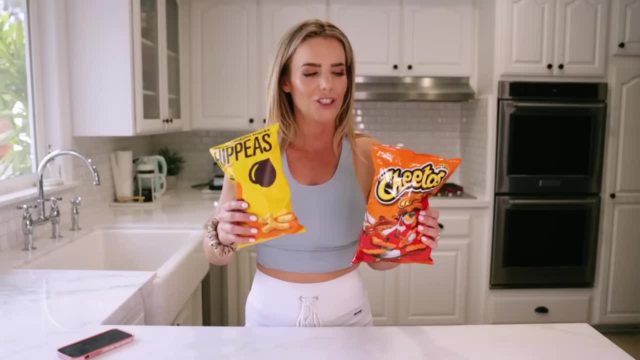 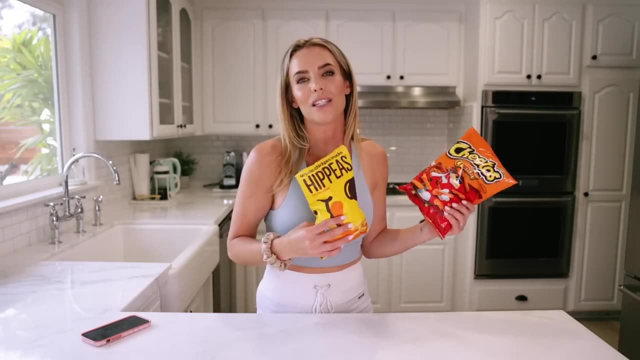 so snack on them, enjoy them, get your cheetah on cheetah cheeto on- watched you guys? but just make a better swap and you can still enjoy those foods and those snacks that you like. again, you don't want to be eating them all day, every day, but you can enjoy them without having all that added junk. 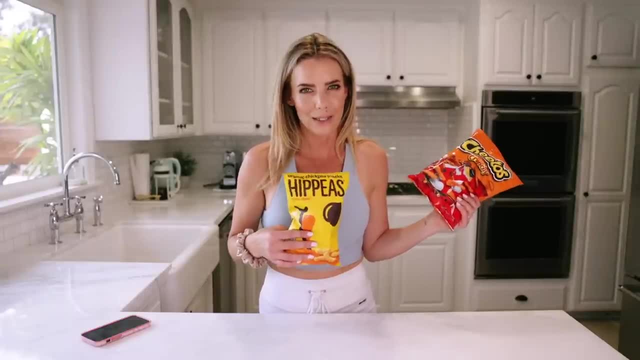 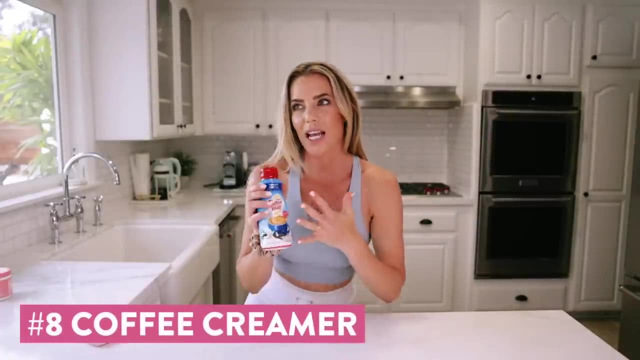 that your body doesn't want and you don't want, especially if you're trying to hit some fitness goals. i used to be a coffee creamer addict, like my coffee was basically white because i would just mostly pour tons of creamer into it because it was so delicious and sugary. um, and it was funny. when i grabbed this one, i was 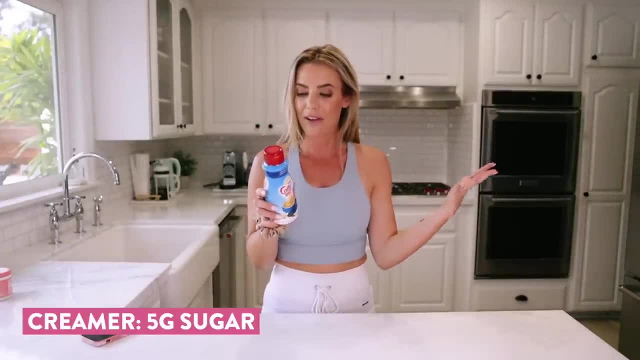 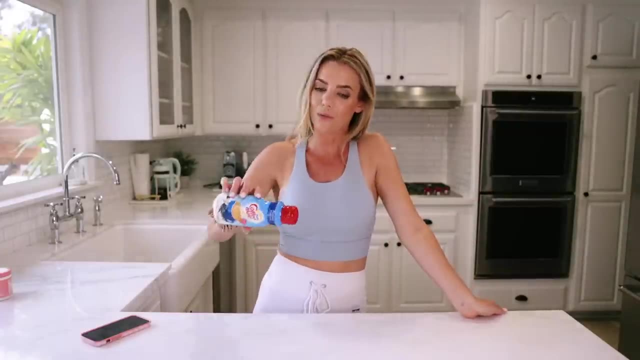 looking at it i was like: oh like, the sugar is not that bad. it's like five grams of sugar, but that's one tablespoon, and i don't know if you measure your coffee creamer, but if you're like me and you're just like, it's probably like four that you end up putting into your coffee to be. 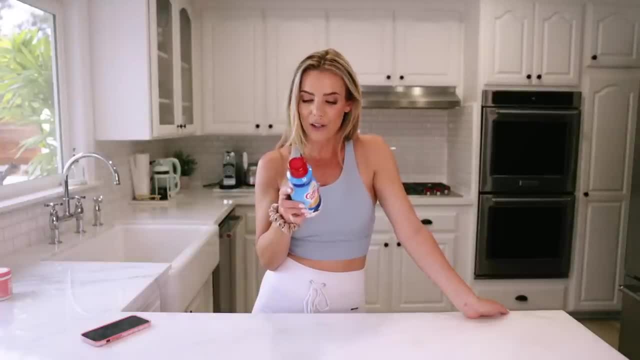 honest. um, that's a lot of added sugar. again, looking at the ingredients, it's just water, sugar, vegetable oil- like why does there need to be vegetable oil in my coffee creamer? that's weird. um, and a bunch of other ingredients, and i'm going to show you how to make a coffee creamer. 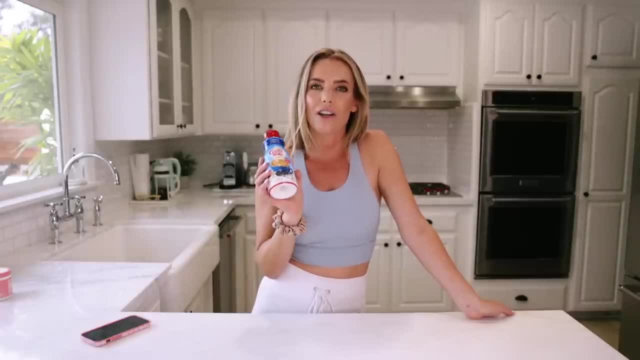 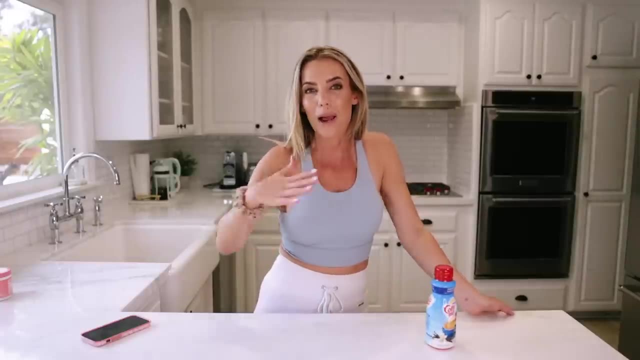 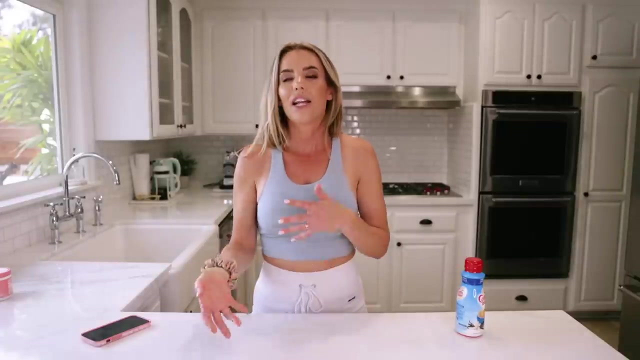 so if you're someone who loves coffee creamer, you want that sweet, creamy yumminess. i get it. but make a swap. so my swap. i went like hard. i went from this to like nothing and just unsweetened almond milk for a really, really long time. then i started like putting a little stevia or monk. 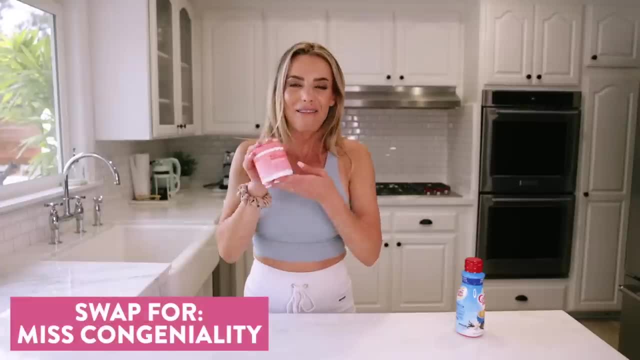 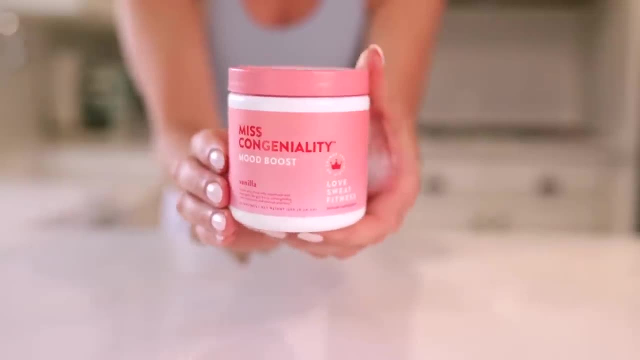 fruit into it. and then now, obviously, as you guys know, i have this congeniality mood boost and this acts as my creamer. so the great thing about this is you can literally put one scoop of coffee creamer in and your coffee will taste sweet and yummy. i think it was coffee made. they used to have this. 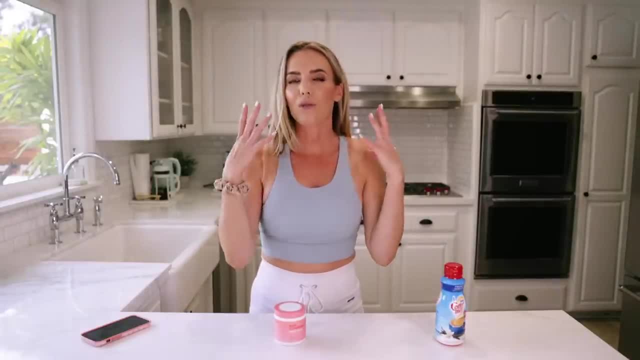 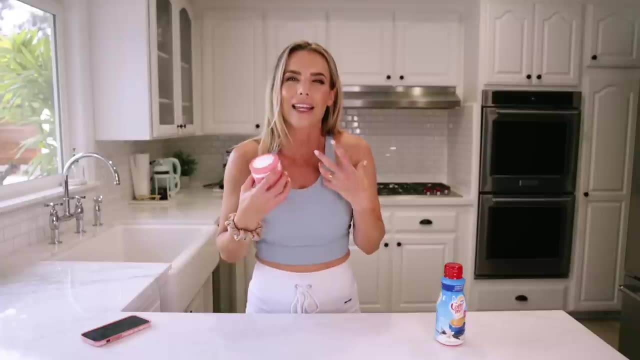 i've talked about. it's like a nutty vanilla flavor. they don't have it anymore, but like it was so good, i loved it so much and that's what this reminds me of. it's like a nutty vanilla, so delicious you don't even have to add milk, but i like that creaminess adding like a coconut milk or almond. 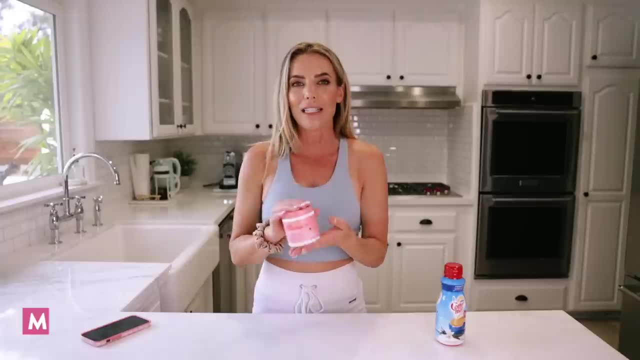 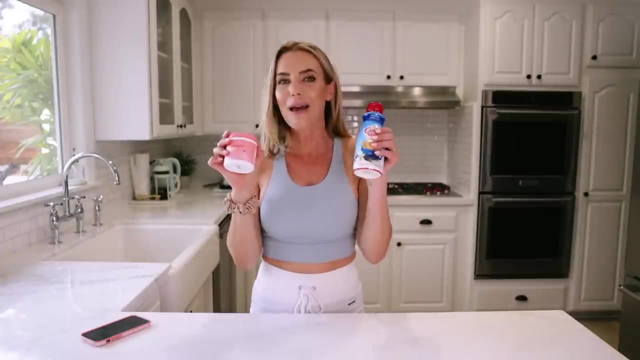 milk or cashew or something to my coffee. so i'll do a little bit of that and my miss congeniality mood boost, which has all the adaptogens, vitamins and minerals to help elevate your mood and reduce stress, and that is the best swap you could ever make for a coffee creamer. so i'm going to show you. 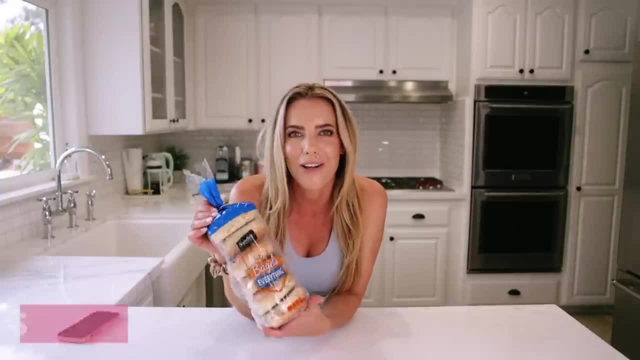 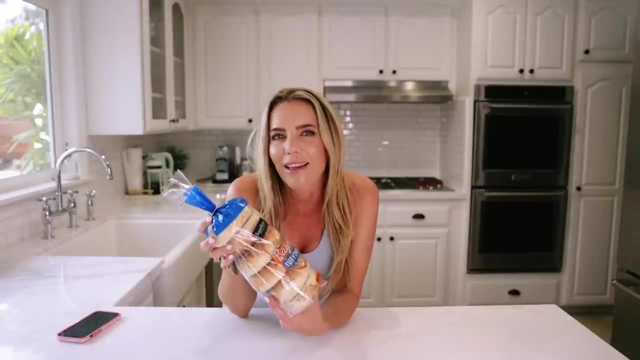 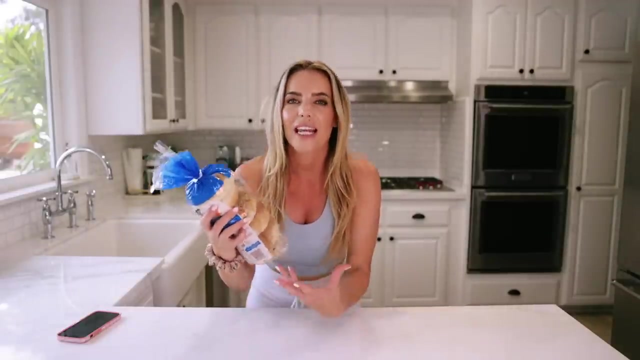 what i ever do for your coffee creamer bagels. um, i don't really think i ate a lot of bagels growing up and then i got into like a big bagel kick a while ago, uh, and i was looking at all the different ones out there. i love an everything bagel. it's so good. and again i need- like we all need- carbs. 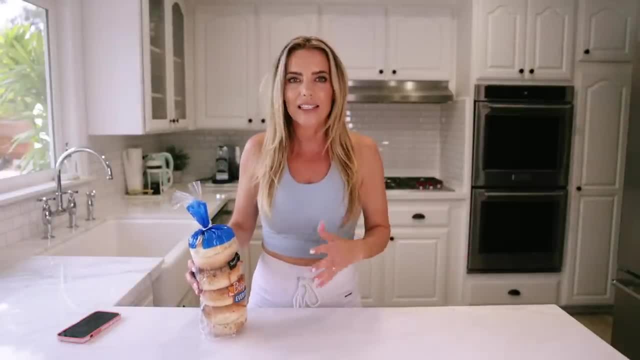 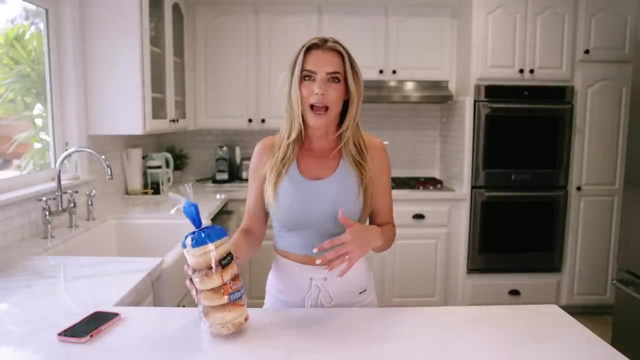 you guys, i don't worry about the grams of carbs that are in things like. it does not matter to me where those carbs come from. come from is what matters. um, so that's what i started to look at, because if you look at like healthier ones compared to like, just you know your typical brand. 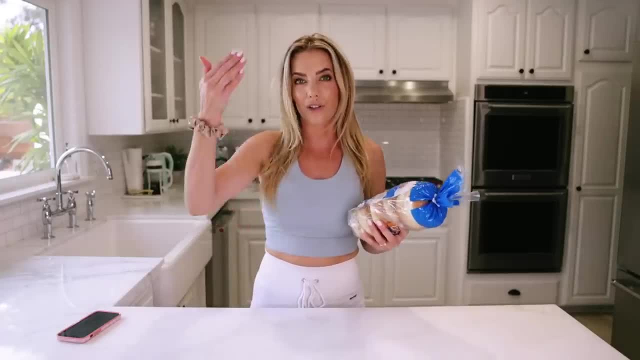 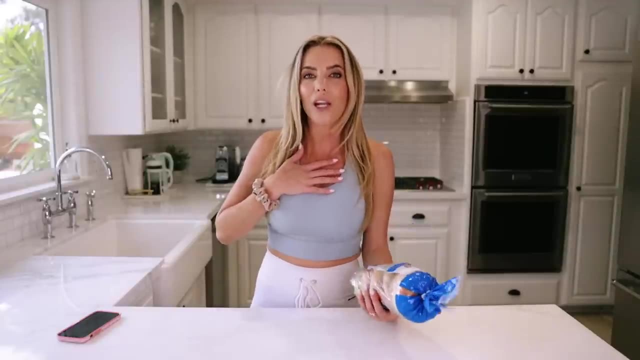 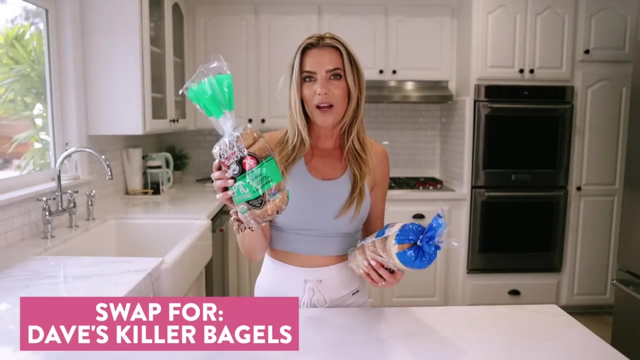 like store brand one. they're pretty much the same when it comes to like your nutritional- like protein, sugar, calories, carbs, whatever- but the ingredients are what really do make the difference, especially someone like me who can be very sensitive to gluten, with hypothyroidism like there's a lot to look at, so these are one of the ones i have been loving. they're not gluten-free. 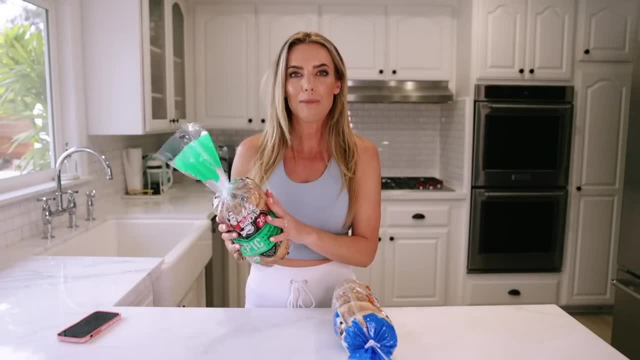 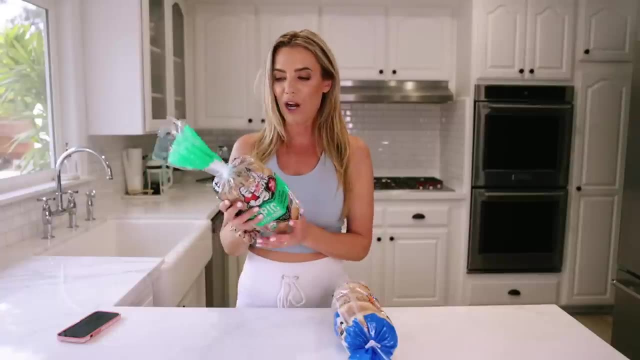 so if you have a gluten intolerance like these aren't going to be your friend, um, but they do not bug me at all. like i can eat them all, my digestion feels normal. i don't get bloated or cramping or anything. so these are epic. everything from dave's killer bread, here's a. 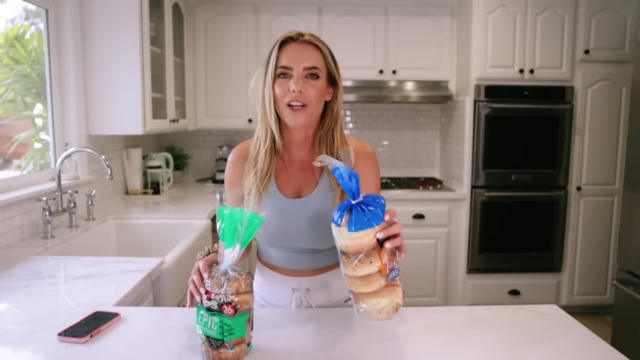 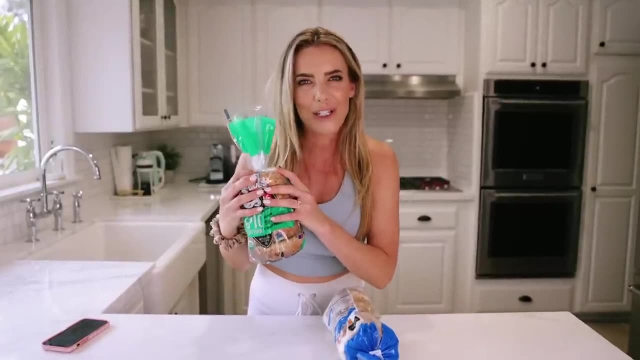 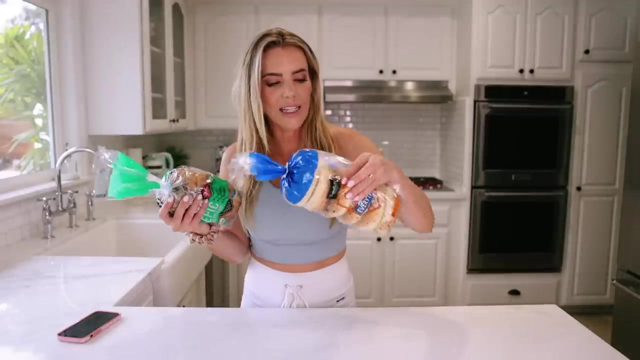 thing. first of all. i know you guys can't feel this, but let me just tell you, these ones feel like really dense and hard. these feel like lovely and squishy and pillowy. so already there's that these are also like covered in seasoning. this one's like kind of like just sad. 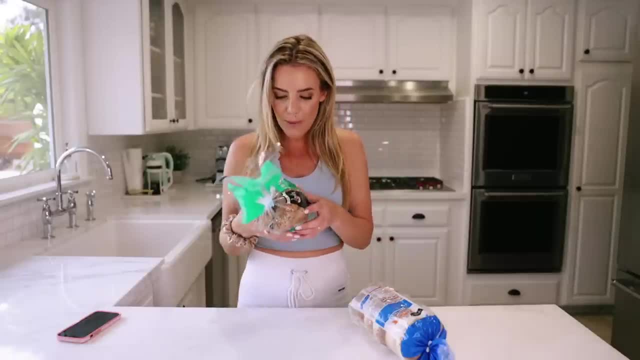 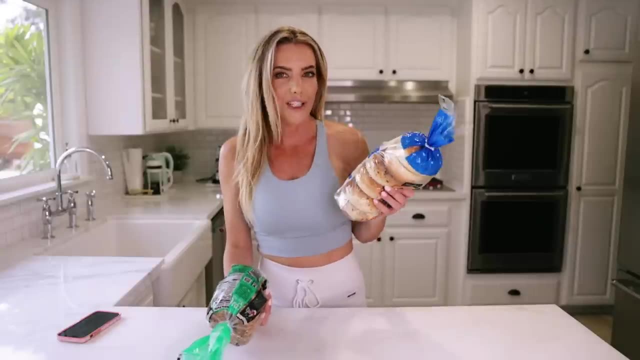 sprinkled on top but like not that much. but then when you talk about ingredients, this one has a really long list of ingredients too, but the quality of what they're made with is very different. so first ingredient here: unbleached enriched flour, wheat flour- um, oh my gosh, lots of things. they. 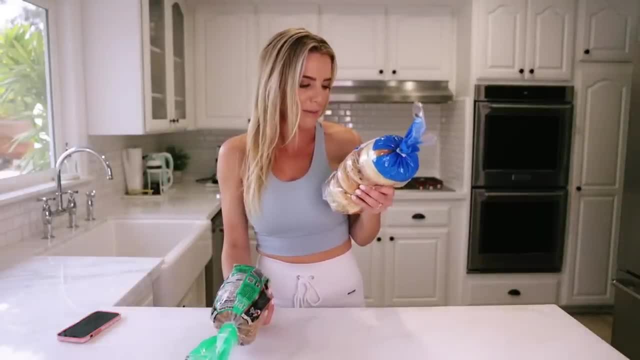 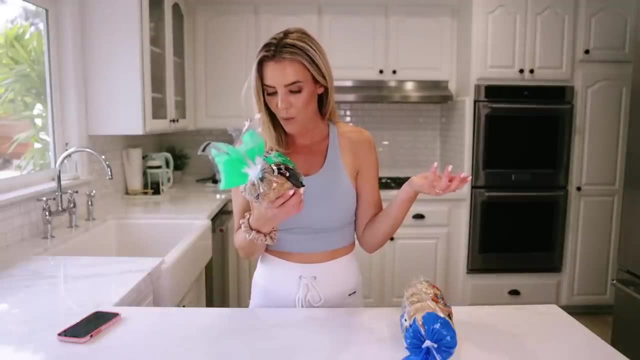 can't pronounce then, like sesame seeds, blah, blah, blah, some gums, i don't even know. there's just a lot of weird stuff in this one. this one is organic wheat, whole organic wheat, flour, water, organic epic seasoning and it tells you everything that's in the seasoning. it's- i mean, it really is like all. 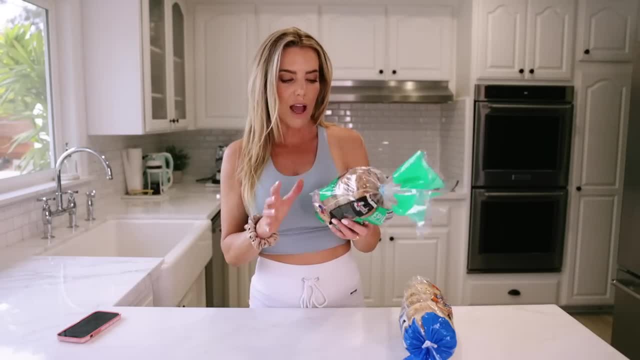 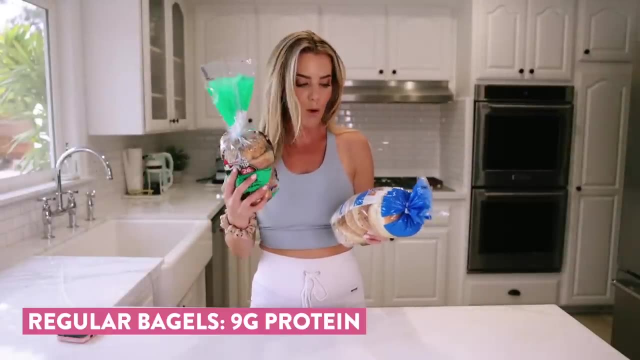 the seasoning and then just like flour, some oil, some water, not much going on like super clean, super good. this is 13 grams of protein, these have nine, so that is obviously more protein here, which is great. um, these have a little more fat, but like who cares, because you're getting so much more stuff. 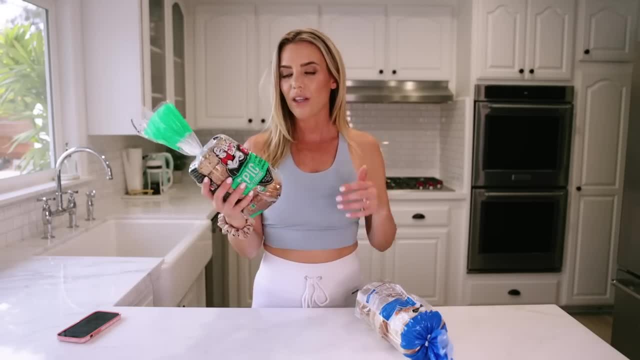 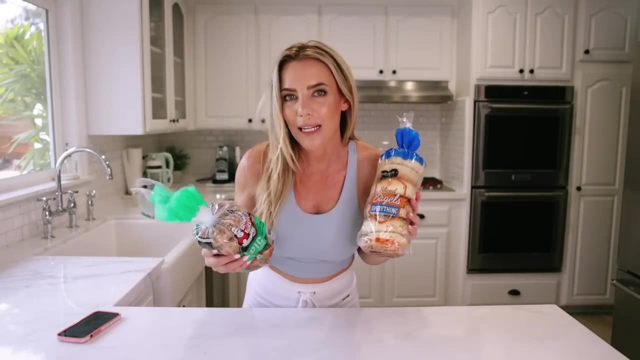 and better quality stuff. so there's probably other good brands out there, but again, i just wanted to get everything from like a normal grocery store. what can you find? so, if you're a person, you don't have to stop eating bagels. you just need to eat ones that are better for you. 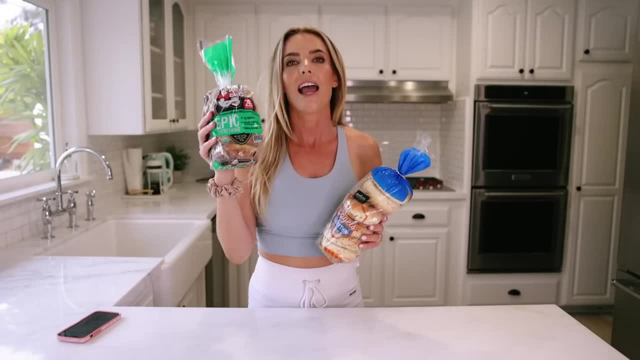 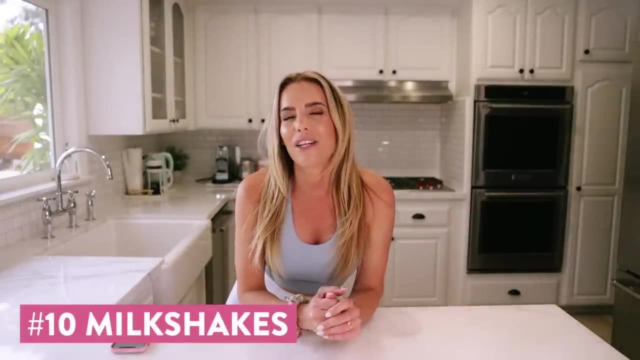 that are going to give you more of those macro nutrients like your proteins, and give you better quality ingredients. and number 10 is a milkshake. you know ryan always talks about how he used to get milkshakes all the time. i i'm not a dessert person, like i'm not a big sweets person, so i was. 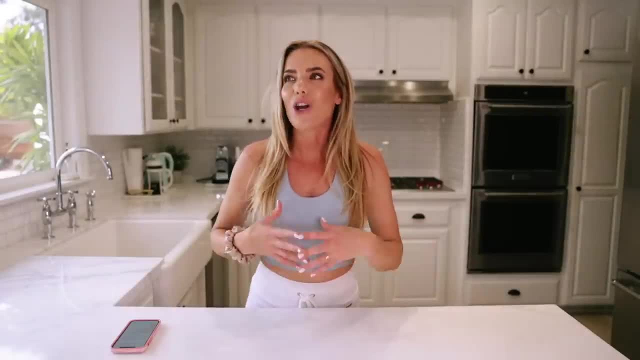 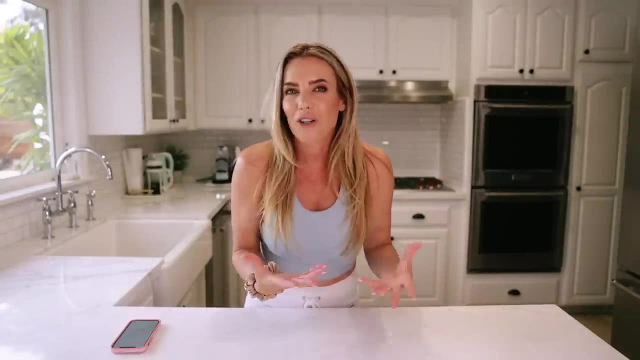 never a big milkshake drinker, but i know people freaking love their milkshakes so i could not bring myself to buy a milkshake because i was like i don't want to waste that money and, like other food, i can donate. a milkshake you can't donate and i just feel like it's a waste of money. 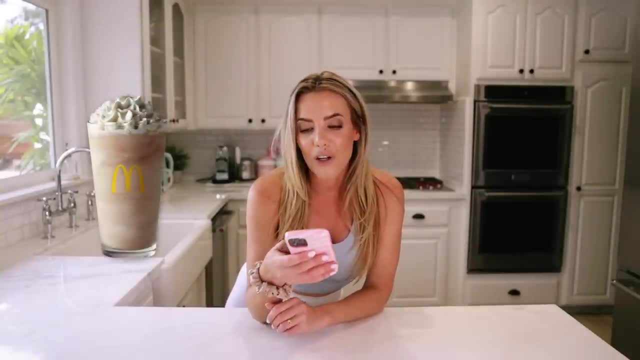 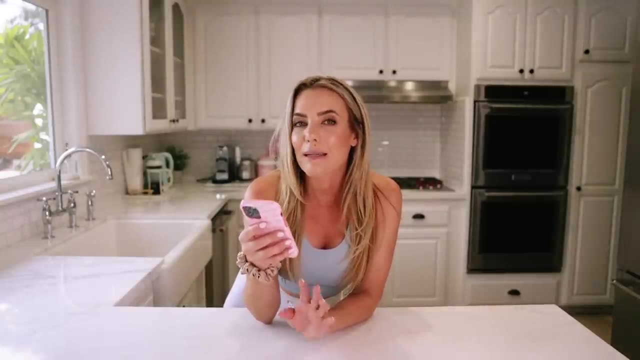 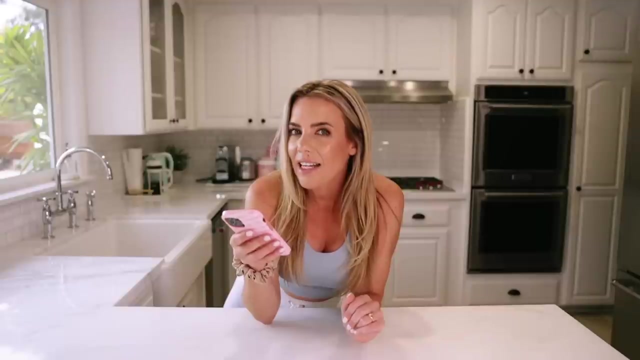 and everything else. so i did pull up the facts for a mcdonald's medium chocolate shake. you guys, i about lost it when i read this. this is a medium, not a large medium. so in a mcdonald's medium chocolate milkshake there's 620 calories. that is a full meal amount of calories like think about. 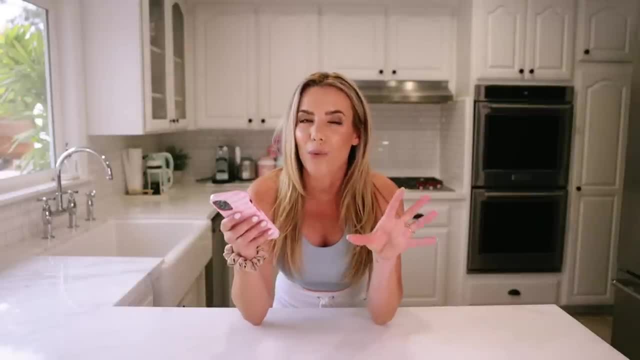 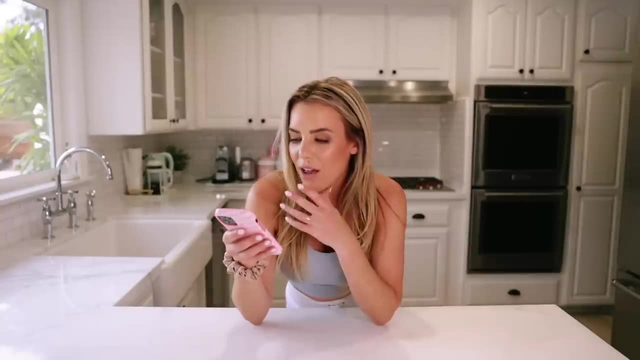 if your day is even based on a 2000 calorie diet, but if you're trying to lose weight you're probably going to have a 1600 calorie range. that's like half your day. that's crazy, okay. so whatever calories it has, sodium doesn't even tell you if it has protein. that's weird. oh, it does have protein. 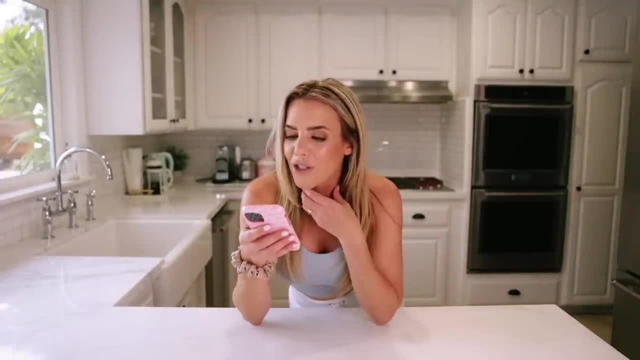 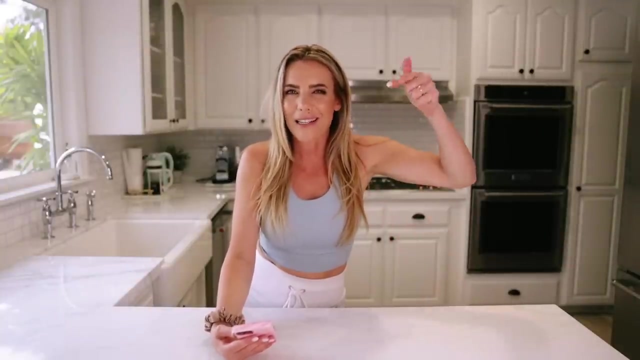 yeah, protein, 14 grams of protein, cool, i guess. um 102 grams of carbs, which is a lot. i said i don't like pay attention to carbs, but over 100 is ridiculous. and 16 grams of fat, fine, but you guys sugar. the sugar you want to guess, drop it in the comments. it has 81. 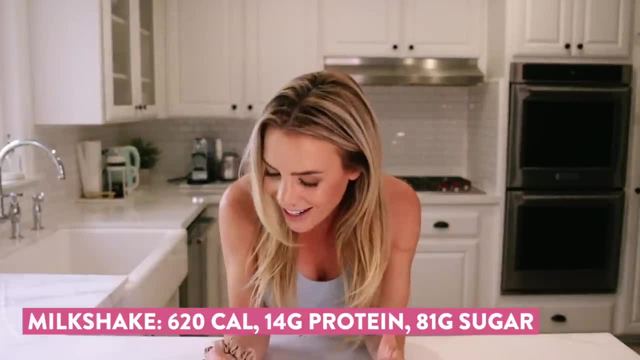 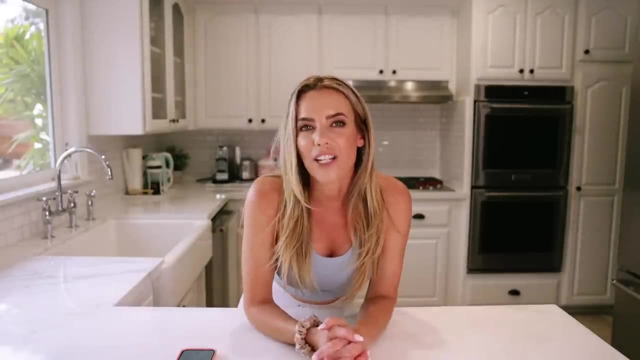 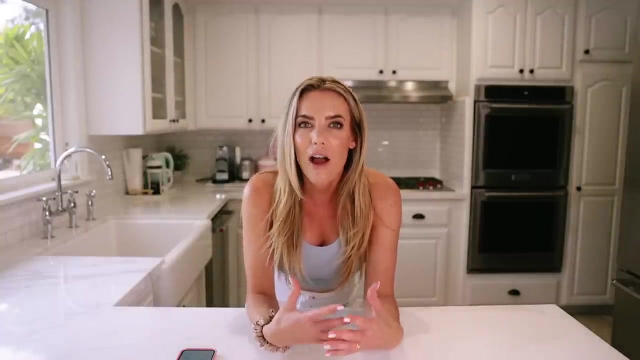 grams of sugar in the medium: 81 grams of sugar. i can't even believe this. moral of the story: never get a mcdonald's milkshake. i, i'm all for things in moderation. that's one that like: no, i'm sorry, no, there's nothing that is okay about that for your body. like talk about mood imbalances. 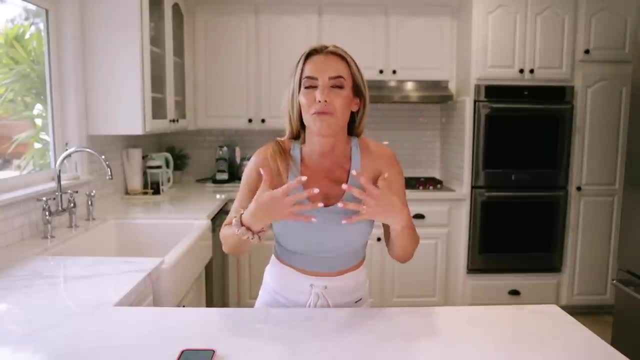 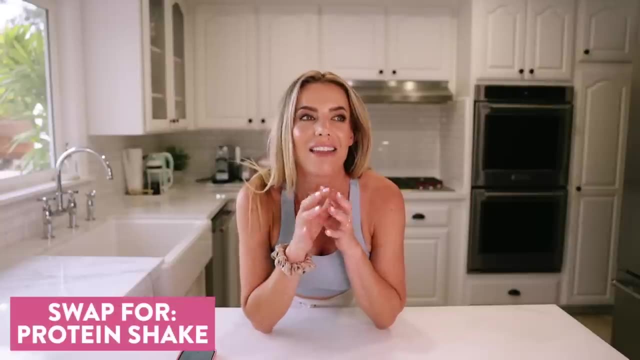 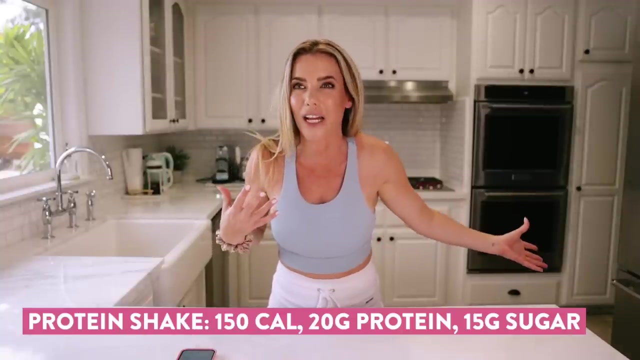 hormonal swings and changes like that, sugar your blood sugar level like holy, no, absolutely not, don't ever have it. i'm gonna make a recipe for you right now: real fast, super easy, delicious, better for you: chocolate shake that's gonna have, like max, probably 150 calories, maybe 200 calories, 20 grams of protein, all the goodness. i'll show you what it is here's. 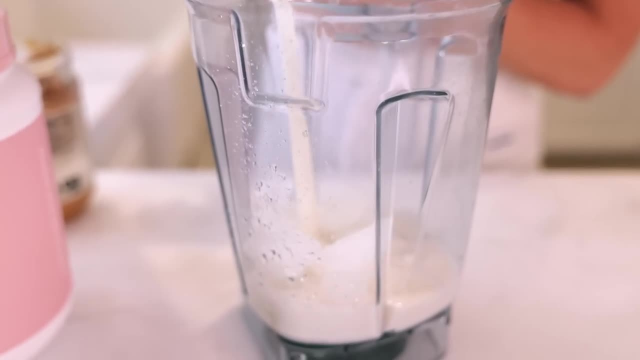 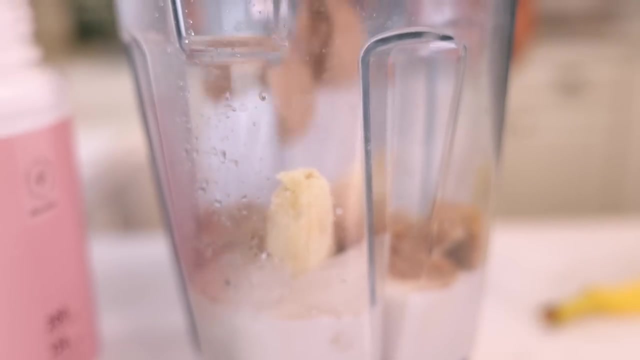 all you need, you guys: lsf, chocolate, plant protein, your natural peanut butter. you now bought a banana that has sugar, but that's okay because it's like 15 grams of sugar and it's from a banana and it's real and it's going to make it sweet and yummy and delicious. and some milk do this. 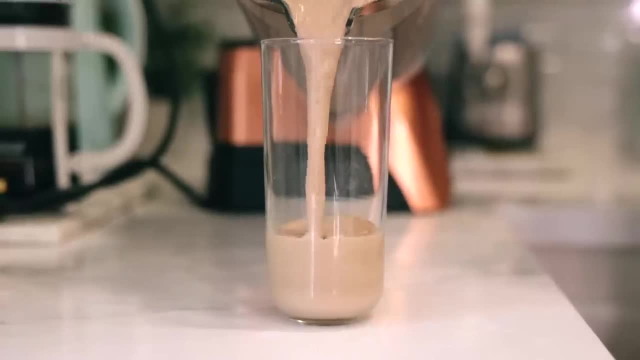 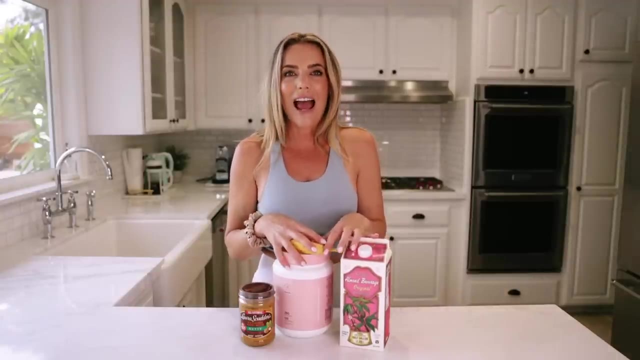 put it together in a smoothie, throw some ice in there and you are going to have a yummy, chocolatey, peanut, buttery, banana protein shake that is going to have over 20 grams of protein. it's going to have all the nutrients you need. you're going to get so many great, healthy carbs. 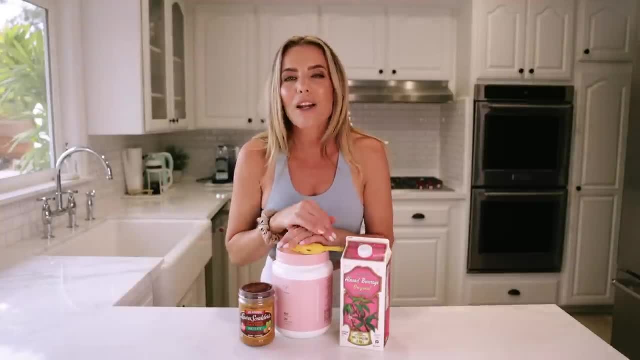 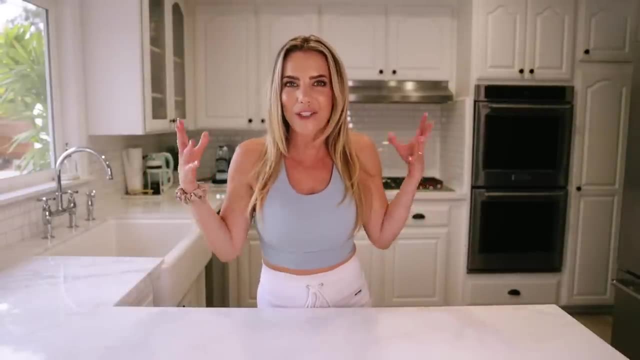 and fats and everything to fuel your day, but it will taste like a delicious treat. that was a lot of swaps. i didn't realize how many 10 really was like once you get into talking about it, but hopefully you guys like this video and found that super useful again and i'll see you in the next video. 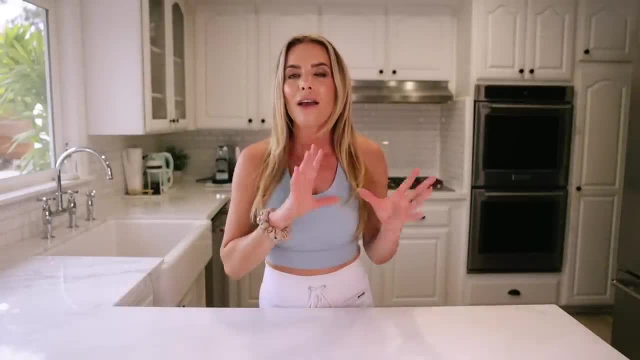 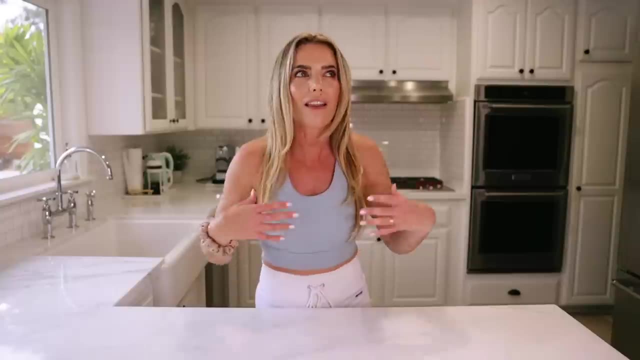 if you are trying to lose weight, if you're trying to just get healthier, making simple swaps like this will make a huge difference in you being able to reach your goals and also just still enjoy life and live life like that is what i did to lose 45 pounds. it wasn't some crazy drastic change. 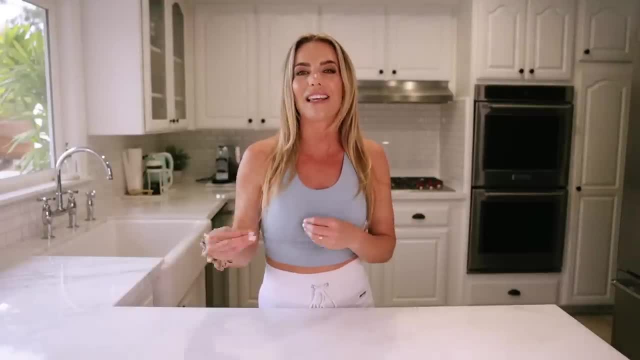 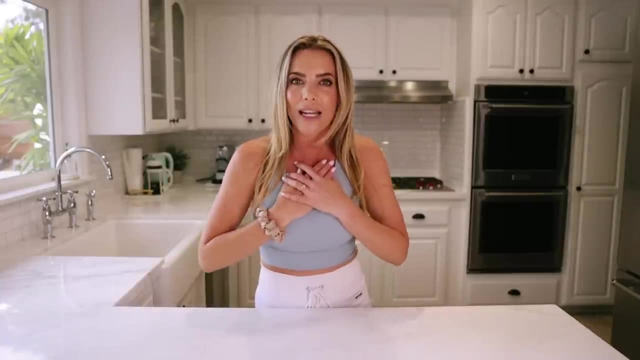 my bagels just dropped. it was just making little swaps like this and over time it makes a huge difference. so if you like this video, hit that thumbs up. it truly means so much to me. it tells me that you want more like this, so i will keep making them.